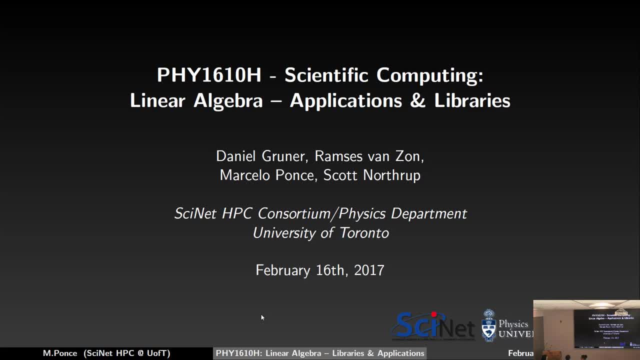 All right, Any questions? from last class, We basically reviewed some linear algebra, a lot of linear algebra. I would say It was like a one-year course condensed in one hour or so- An hour and eight minutes actually. Any questions about that? No Good, 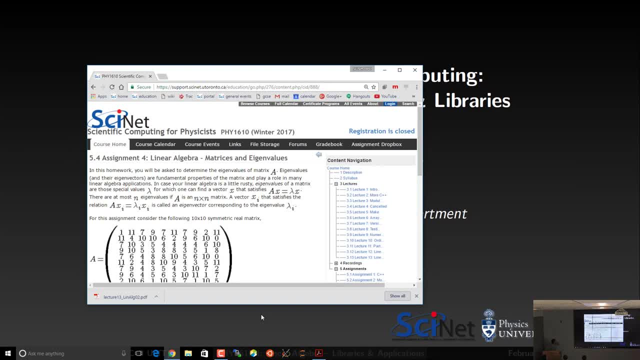 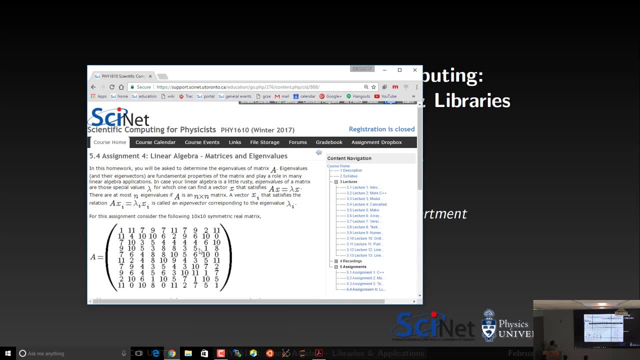 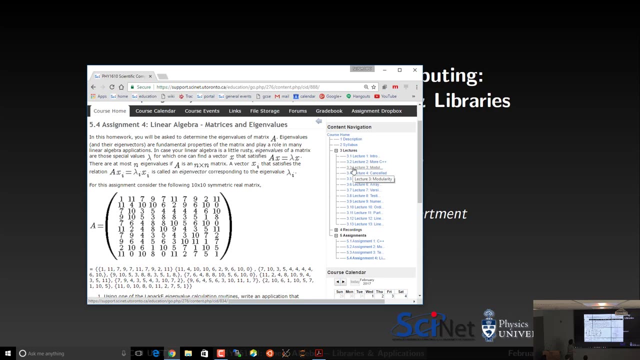 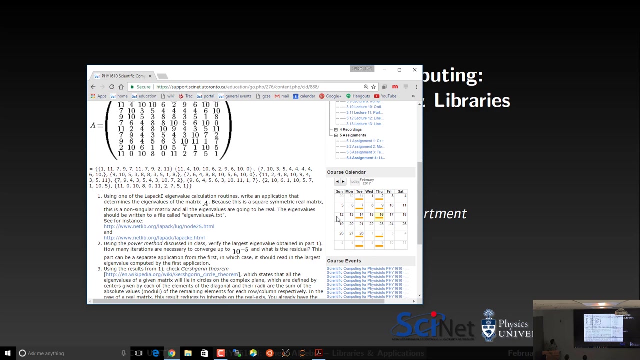 Just to let you know that the assignment was posted and, of course, as it couldn't be any other way, it's about linear algebra. So you have that nice symmetric 10x10 matrix there. So the problem asks you to compute the eigenvalues of the matrix first using one of the libraries that we are going to be discussing today. 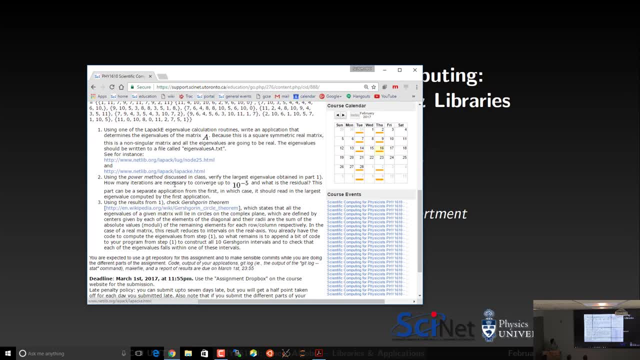 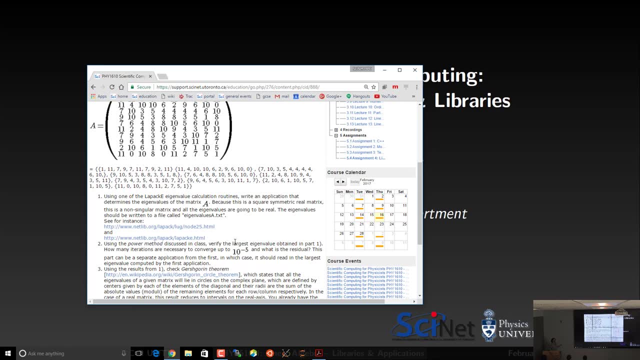 and then the second part, to compare those with the power method that we discussed last class, And the power method you will have to implement from scratch. Of course, you can also use linear algebra routines for doing whatever you have to do in the power method. 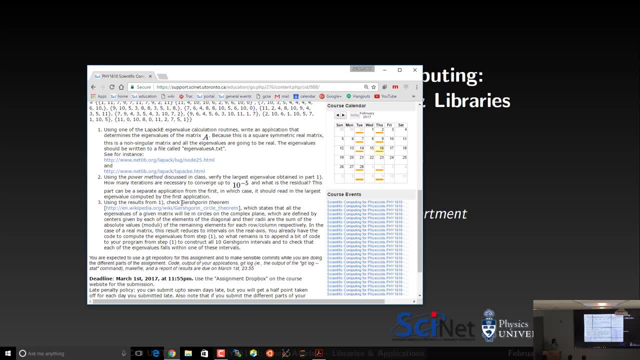 And then the last part is to use something that is quite neat, I would say, which is the Gersh-Coring theorem. How many of you have heard about the Gersh-Coring theorem? Yeah, let me, Oh, okay, Excellent question. 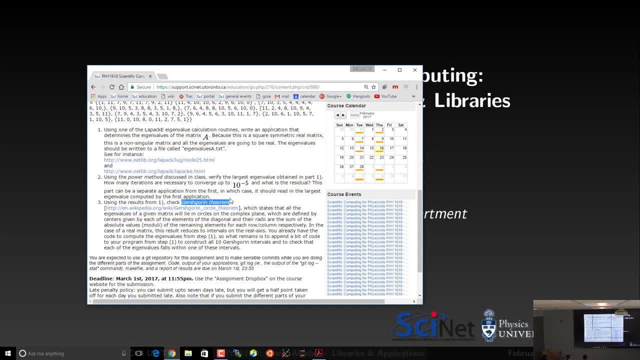 So now I can talk about the Gersh-Coring theorem. So the theorem applies for any kind of matrices And we were discussing- and in this case it's a real matrix- But the theorem applies also for complex matrices. So when you compute the eigenvalues of a complex matrix, 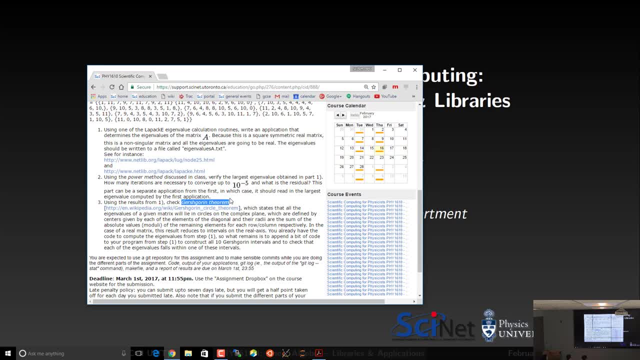 your matrix, The eigenvalues are on a plane, in the complex plane. But when the matrix is real and when the eigenvalues are real, your circles reduce to intervals only on the real axis. So if you have an eigenvalue, let's say 1i or i1, being i the imaginary unit. 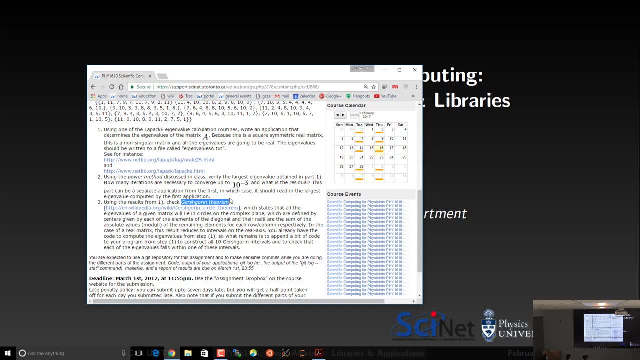 it will lie in that plane right And the circle will be something that is the addition of the. The theorem works for columns or rows, So it will be the addition of all the remaining elements in the row or the column. That's the radius of the circle. 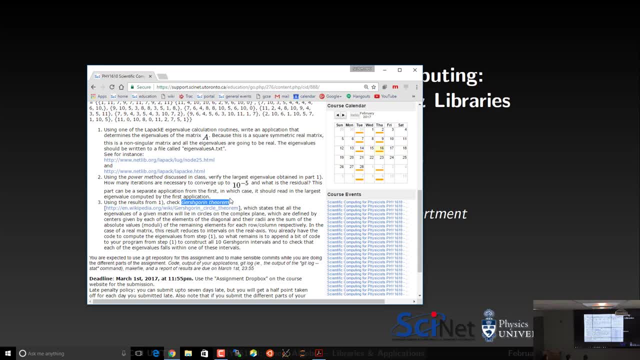 Now, if your matrix is real, like in this case, and symmetric even more, your eigenvalues will be all real And they will be only the real. So this is the real axis, the imaginary axis. So in this case, these are intervals. 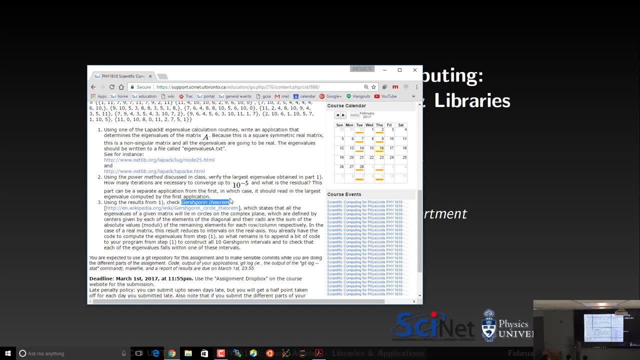 Okay, so the theorem is general enough that it applies for complex eigenvalues. So that's why it says So that's why it says Circles on the plane, but in this particular case are intervals on the real axis. 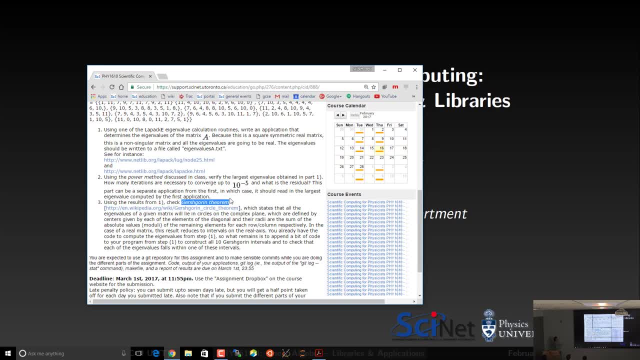 Okay, If you want to draw the intervals for the circles in the complex plane, you're welcome to do it. Okay, So I just wanted to mention this And I finished due on March 1st, so not next Wednesday because it's reading week, but Wednesday after that. 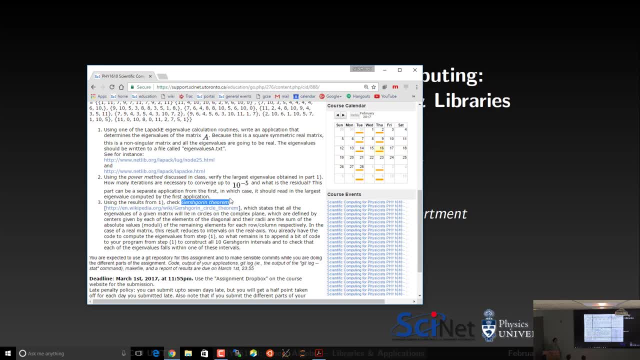 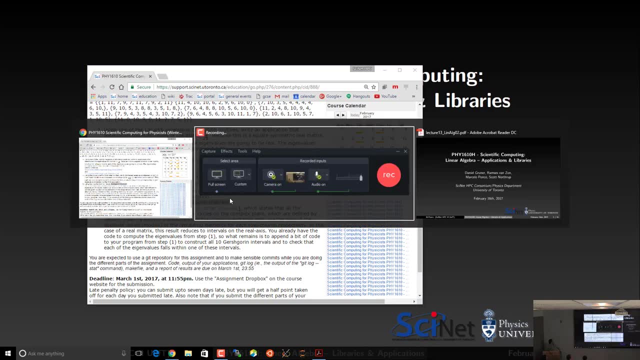 Okay, And I finished due on March 1st, so not next Wednesday because it's reading week, but Wednesday after that. Any questions about this? Any other questions about this? Was this clear? Yeah, All right. So let's take a look then at the utilities part of the linear algebra. 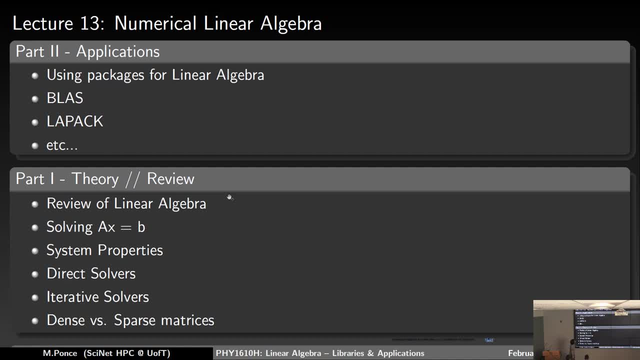 So last class we reviewed a bit of theory. Today we're going to be talking about the packages that you can use for actually doing some numerical linear algebra. In particular, we're going to focus in two: BLAS and LAPAC. 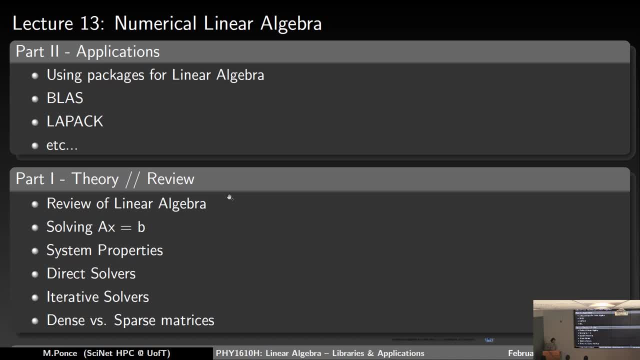 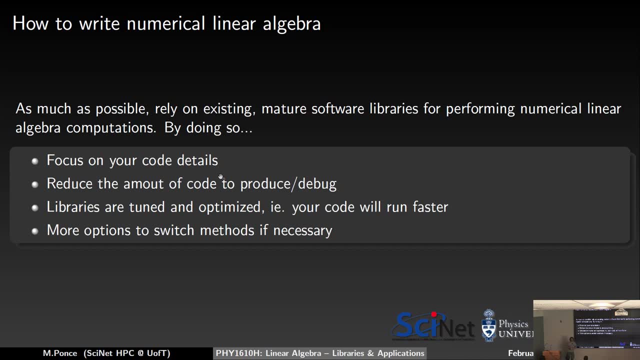 We're going to talk a bit more about other ones, But these ones are So we mentioned this also- last class. There are many techniques and many methods that you can implement for dealing with linear algebra, either for solving the linear systems, for computing eigenvalues, for doing matrix decomposition. 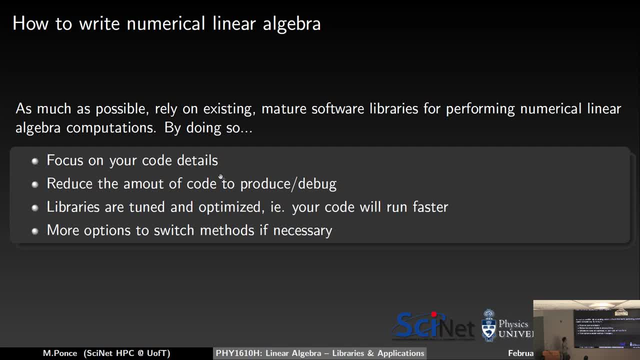 different kinds of things. right, The thing is, these techniques have been in place for a long time and the libraries that we are going to see today, they have been developed for a long time. So many of them have been optimized until the last line of code. 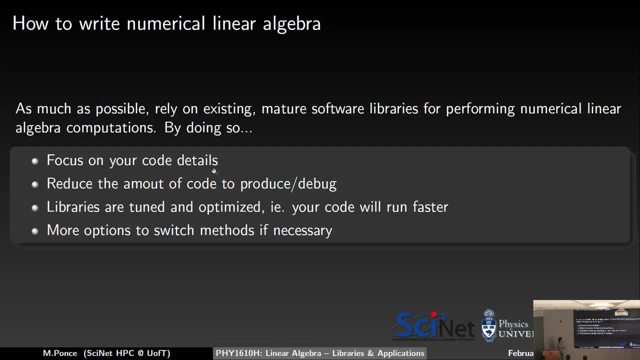 Every line of code has been thought for people or by people that actually deal with that all day, and it's their profession basically to deal with that. So our suggestion is: whenever there is a library there that has been tested, that has been proven to be optimized until the end, just try to use it okay. 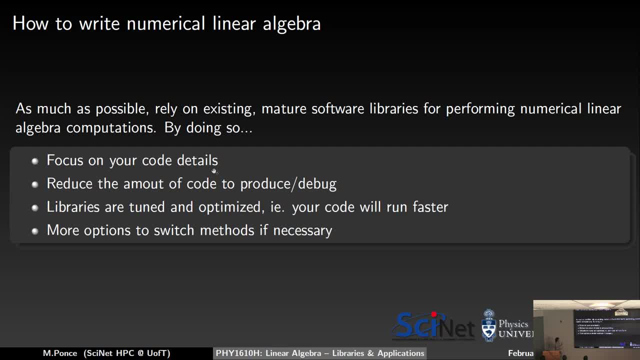 You may have to spend some time learning. So many of them have been developed for a long time. So many of them have been optimized until the last line of code. you will see- I know we'll sugarcoat this for you. 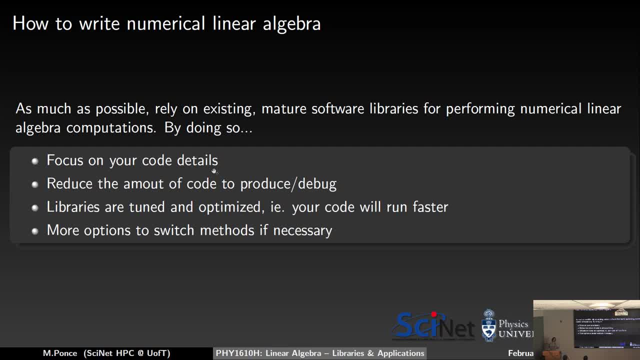 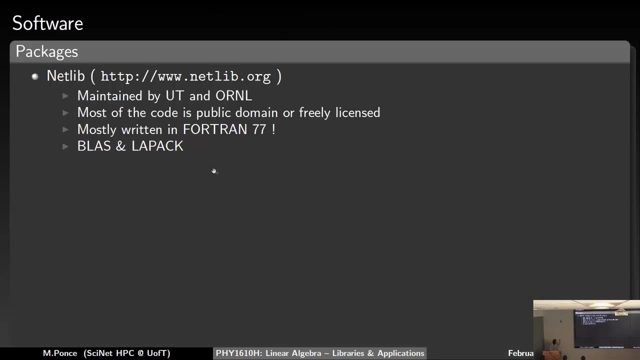 some of the routines are kind of cryptic and you need to get used to the terminology and the nomenclature, basically. but it's worth to learn that and use these tools that have been optimized until the last line of code. Okay, which packages are available there? 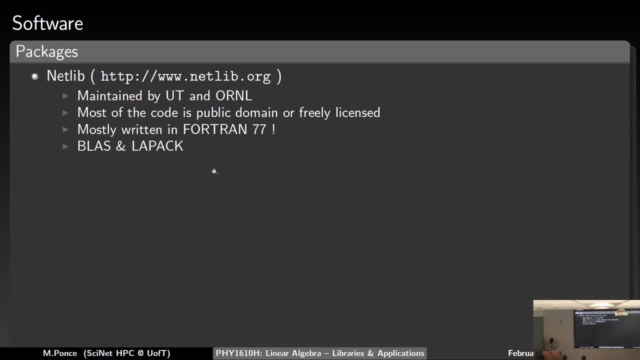 So one of the- actually this is kind of a repository, as you wish, or an interface- is the Netlib that contains information for BLAST and LAPAC. Mostly this is written in Fortran 77, which is quite old, as you can notice. 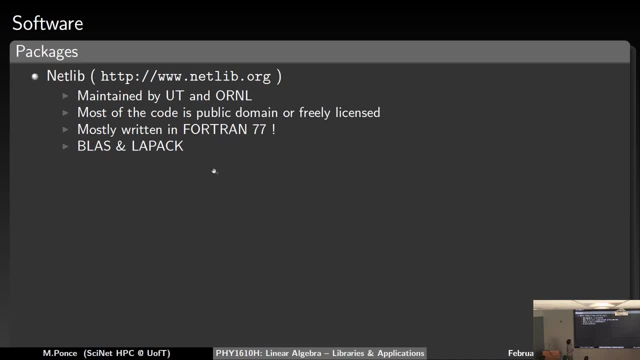 but they have interfaces for C or C++. Most of these codes are public domain or freely licensed, so you are free to use it. It's maintained by University of Tennessee, I think, and Oak Ridge National Labs. The other one, Petsy, is also maintained by one of the national labs. 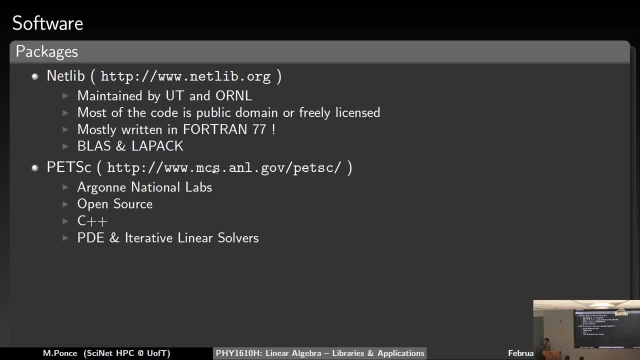 This happens a lot like. I don't know what is the deal with the national labs in the States, but they like to compete each other. They have a visualization package called One Visit and The Other Paraview. Each of them is maintained by one of the national labs. 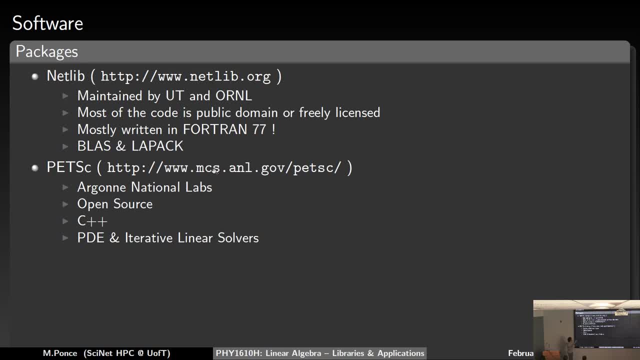 and their goal is to basically do the same. so I think it's some kind of friendly family competition going on there. This may be kind of the same. The only difference is that Petsy is well, it's open source as well, but it's C++. 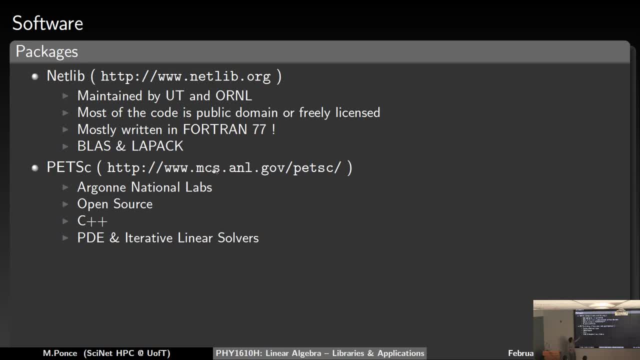 So that's the only difference. I think it's a little bit different. I think it's a little bit more complex, But I think it's a little bit more fun, and I think it's a little bit more fun. So, yeah, I think it's a little bit more fun. 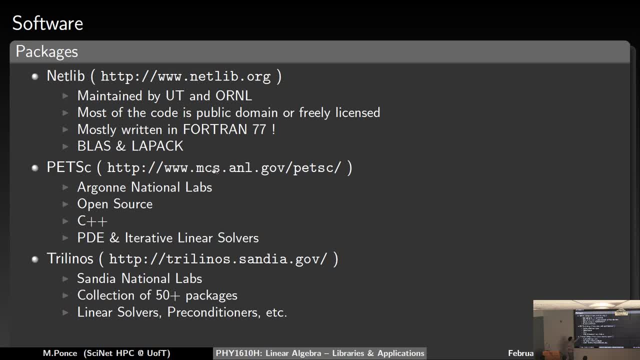 So, yeah, I think it's a little bit more fun. I think it's a little bit more fun. And then there's the other one, which is also maintained by a national lab. It's called Trilinos. Trilinos is a collection of 50 plus packages. 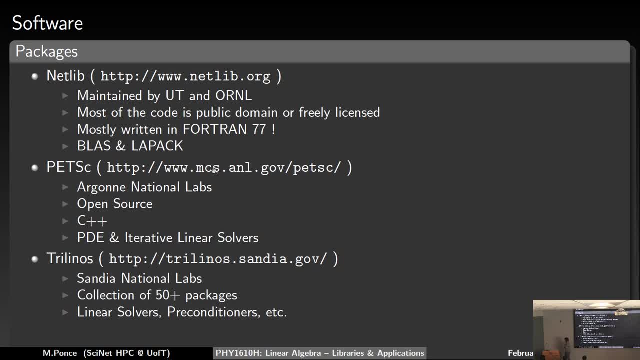 maybe more now- which include linear solvers and preconditioners- Remember, we talked about the conditioning number last time- and the whole- you know the whole package, and the whole package, and the whole package has a very high field of preconditioning research. 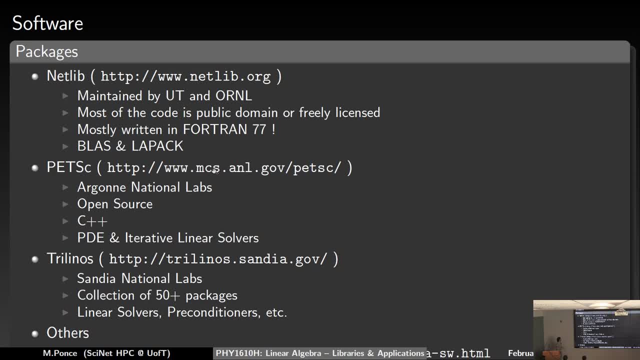 So these guys can do that for you, And for sure there are many others. If you look, there are parallel versions of, for instance, Laypack. It's called Scalapack. One interesting thing, though, is that even when this library 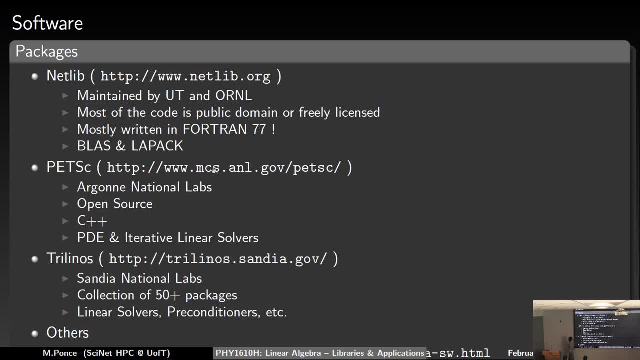 is that, even when this library has been developed and optimized, especially the parallel versions, to get you the best performance? I don't remember the name. Remember when we went to the Compute Ontario research day two years ago. there was someone presenting a shift in the paradigm that people are trying to use to solve these linear algebra. 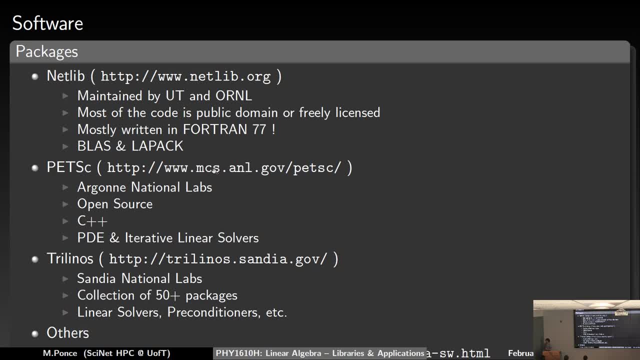 operations And the bottom line is that nowadays, computing on the node is cheaper than sending information on the net or passing information to your next node. So many operations now. or the approach is to switch instead of sending information out of the node. recompute things on the node. 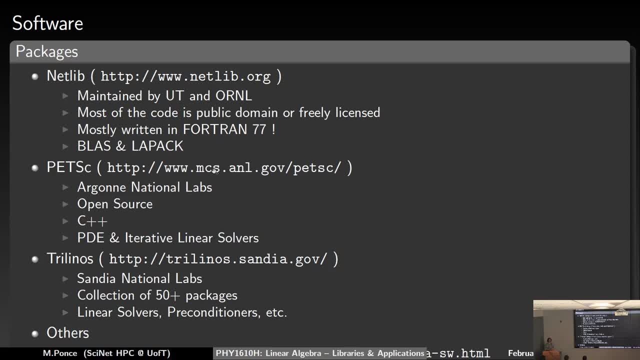 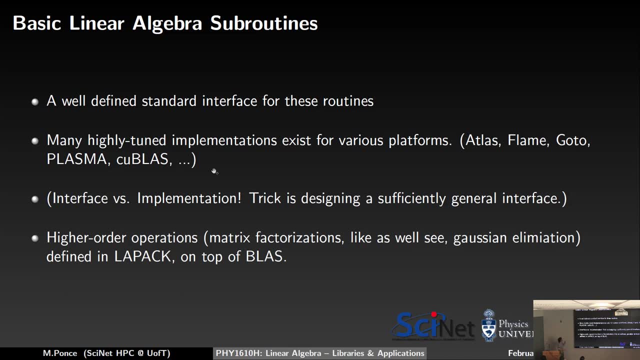 So some of these libraries are being rethink in terms of that, Anyway. so let's take a look at BLAST. So BLAST stands for Basic Linear Algebra Subroutines. It's a standard. It has been for a while. It's highly tuned for different platforms. 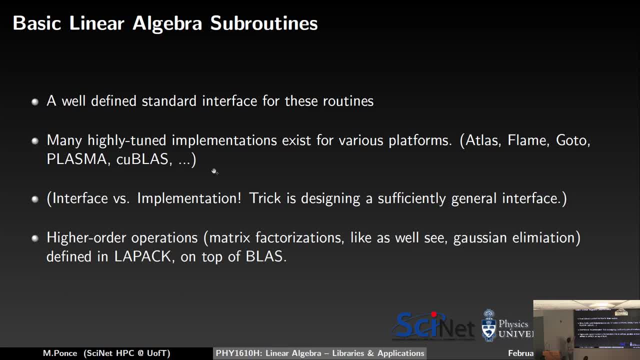 You may be familiar with some of them. By the way, there are issues that are interesting. in using GPUs, NVIDIA has a nice implementation called kubelast, which is CUDA BLAST. There's a difference between the interface and the implementation, and this is something. 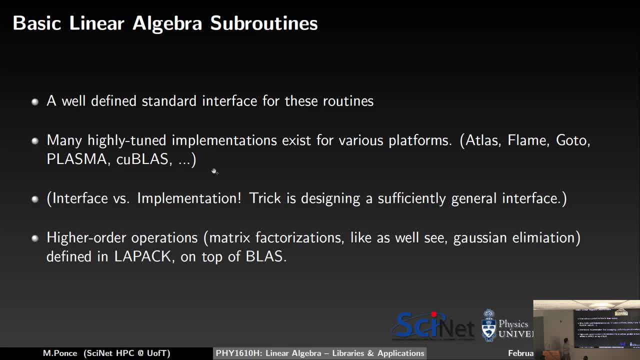 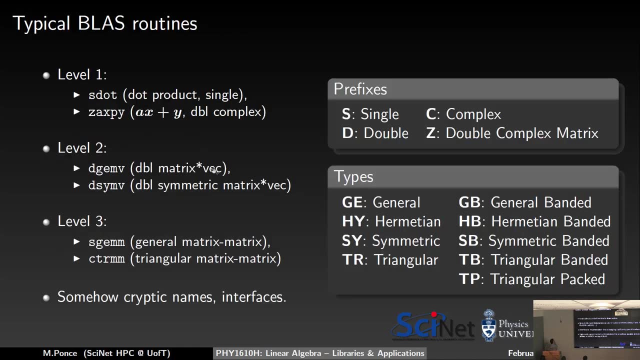 that we are going to see more in detail in a second. It includes a lot of things. It includes high-grade order operations like matrix factorizations and Gaussian elimination. Those are defined in LaPAC and on top of BLAST. So let's take a look. 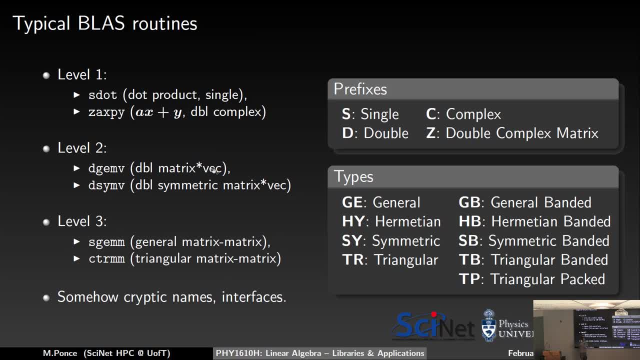 So this categorization- and this is where things start to get a bit more cryptic in terms of names and how to call the routines- There are basically three families or three levels of different routines and you will see something similar. So the first level are, and each level is like gaining in complexity in the sense of 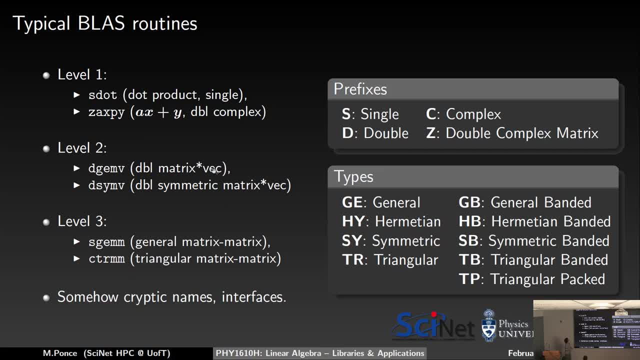 which operations you can achieve or which structures you deal with. The first level implies dealing with dot products, For instance, S? dot is the single dot product. SASP is solving the linear system AX plus Y, So SASP, the set stands for double complex. 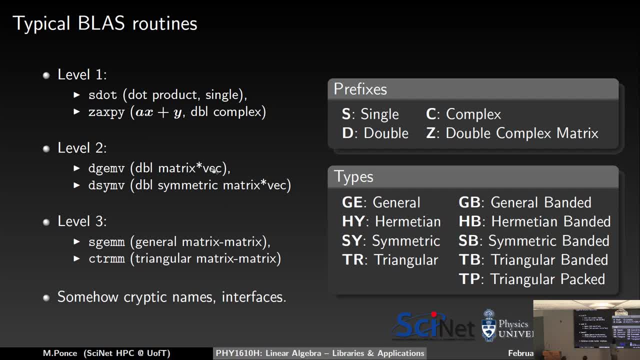 So we are going to see- We have prefixes in front of the names- where S is single, D is double, C stands for complex and Z is a double complex matrix. So S is a single variable with a dot product between two vectors. 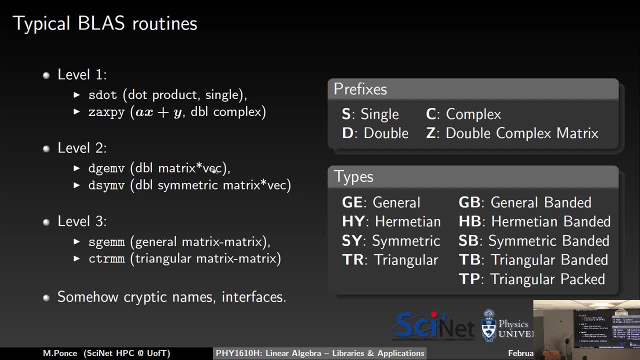 SASP in that case is a double complex matrix solving this linear system, AX plus Y. The level two type of operations or routines are Matrix vector multiplications. So initially you have vectors, basically level one. Level two is matrix vector and here D stands for double. again, 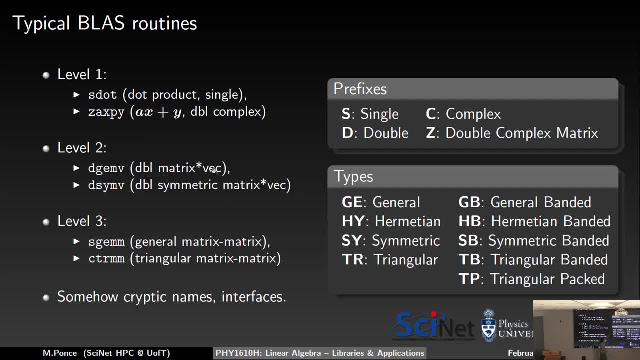 GE in this case is now a general matrix. So remember we spent a good amount of time last class discussing that: the structure of the matrices, Different kind of matrices like upper triangular, lower triangular, banded matrix. So we are going to look at the structure of the matrices. 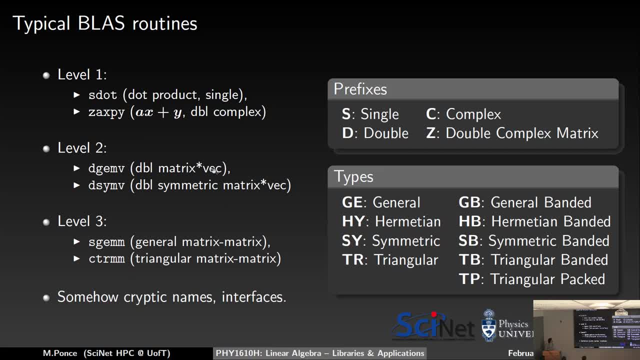 We are going to look at the structure of the matrices. We are going to look at the structure of the matrices Diagonal, So these routines or these libraries knows about all these types of matrices and can take advantage of that structure. So it's always a good idea, if you know the type of matrix that you are dealing with, to 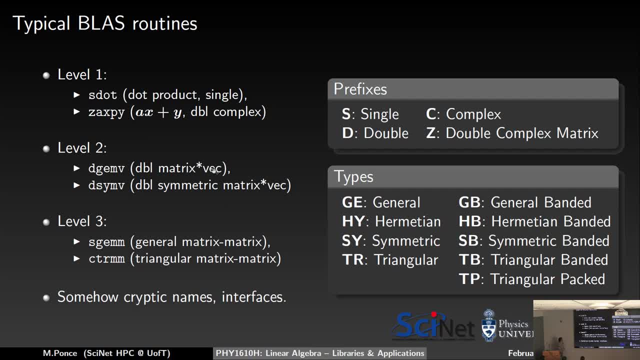 use the appropriate routine for dealing with that specific matrix. So the types that we may have are general, where there is no specific structure underlying Hermitian, symmetric triangular, triangular, Triangular banded, triangular packet, Hermitian banded and general banded. 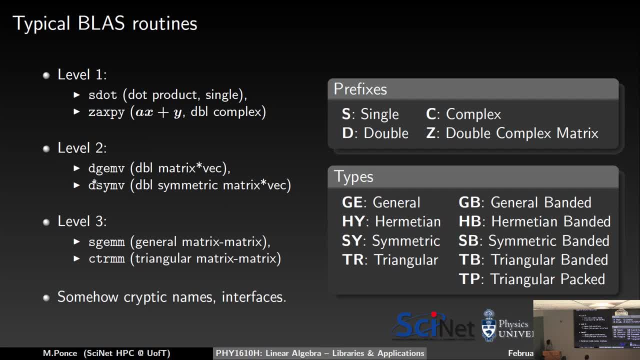 So now you can specify the type of. so you specify the type of variable that you have, and then the type of matrix that you have and finally the operation. So in this case it's always matrix vector multiplication. So that's the MB: matrix vector multiplication. 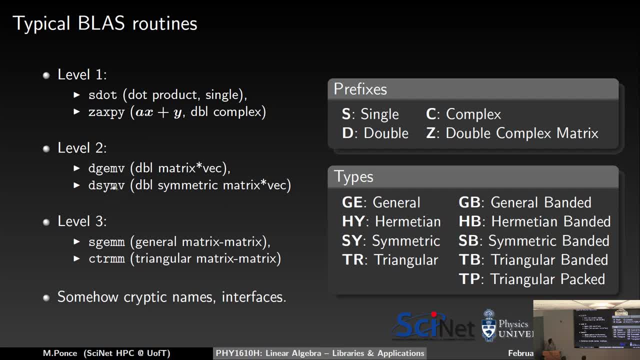 So here we have a double general matrix vector multiplication. So that's the MB matrix vector multiplication. Double symmetric matrix vector multiplication. Double symmetric matrix vector multiplication. Double symmetric matrix vector multiplication. The final level- level 3, stands for matrix-metrics operation. 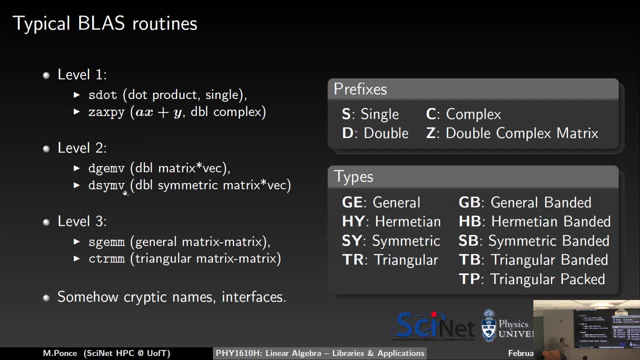 So we start with scalar vector, vector matrix and matrix-matrix. That's the level 3.. And again the nomenclature is kind of the same. So you have a single general matrix-matrix- multiplication, or a complex triangular matrix-matrix. 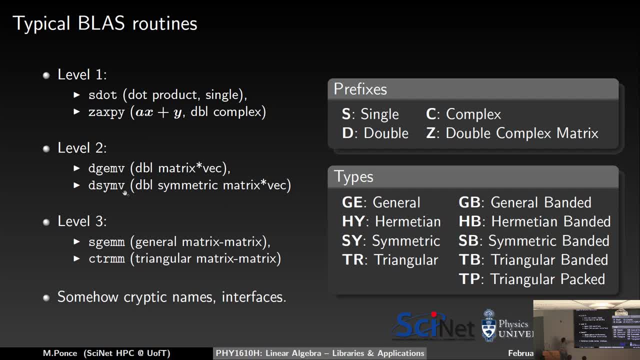 multiplication. So those prefixes of those names are going to specify the routine but also have information about the type or the structure of the matrix that we want to use. As I said, these are somehow cryptic names. You get used after a while. 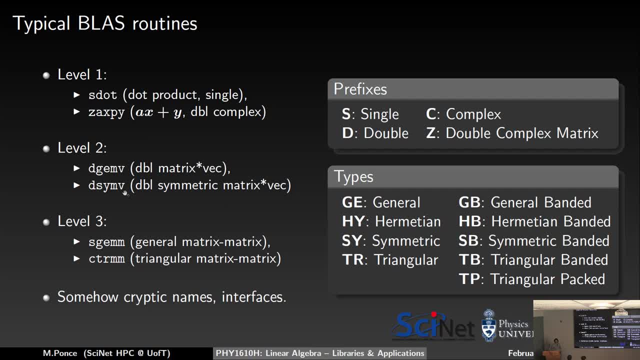 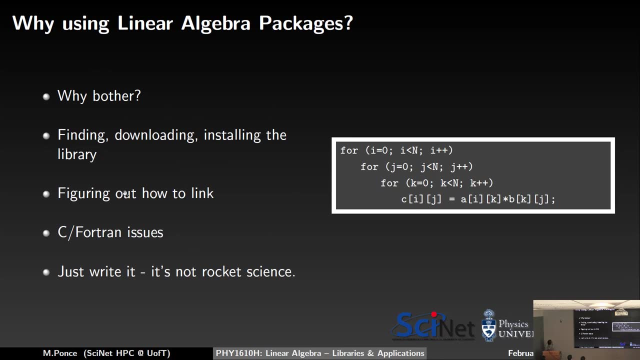 But it's good to know, and it's good to try to remember or at least look at the names and the type of matrix that you're dealing with, in order to know which is the best routine to apply for each case. Okay, so this is a kind of teaser slide, but why bother using these libraries? 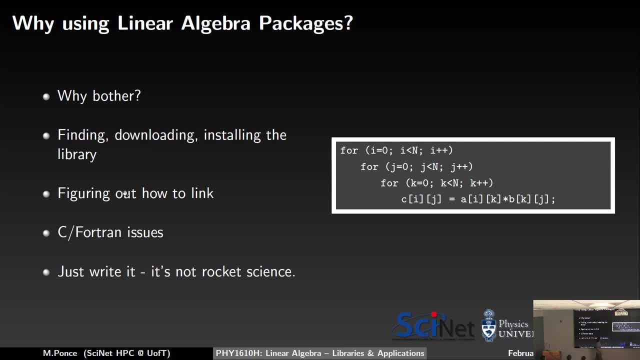 I think I mentioned this at the beginning. but if you think about this, in the worst case you will end up doing these kind of operations, right? Three nested four loops where basically all that you want to do is compute your final result, like a matrix-matrix multiplication. in that case, right. 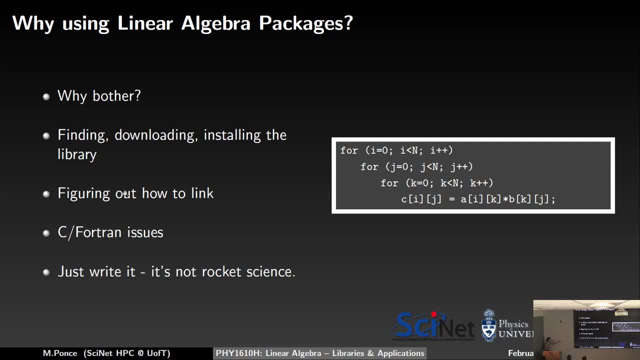 If you prefer, instead of doing that, implementing your own codes, your own routines. basically, the opposite will be okay. if I have the libraries, I have to find the libraries. to install the libraries sometimes implies Compiling most of the times. 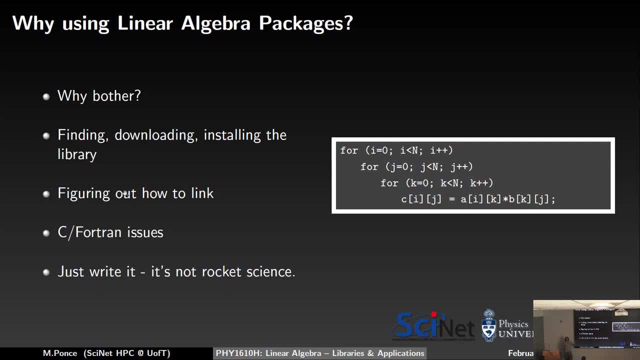 Figure out how to link with the libraries. Most of these libraries I told you about are, at least Blast is Fortran, so there are C Fortran issues that we're going to see in the examples. So the question is, why just not write it and use our own routines? 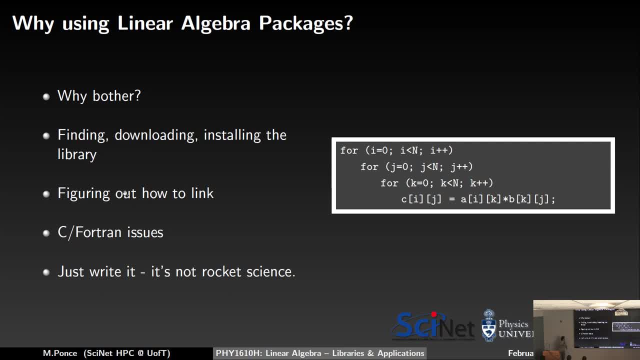 In addition to the argument that I told you about the debugging that has been out for a while now, is the fact that the performance that your code is going to perform, the performance that you're going to get in every single step right. 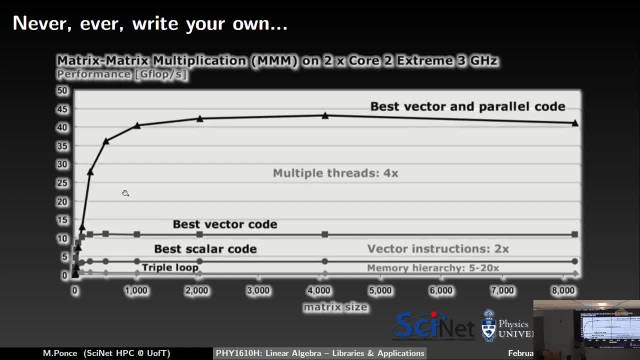 Is going to start to change? Is going to start to change Or is going to be a new step? are going to get in your best implementation or the best implementation that you can achieve with a simple loop kind of matrix multiplication doesn't compare with the best vector and 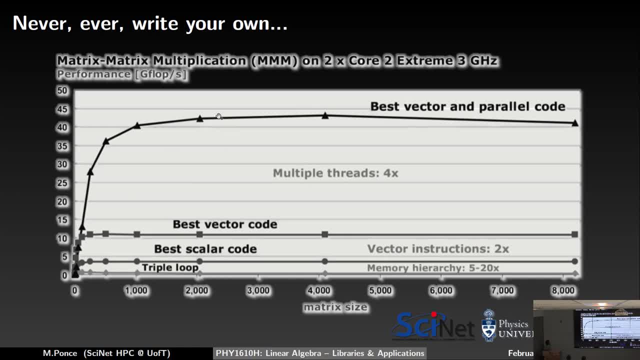 parallelist code that you may achieve. So this is a factor of what file is and this is performance, like Shiga float operation points per second, And this is just a matrix-matrix multiplication. So this is a two-core experiment. I think it's quite old, so this means these numbers may have changed. 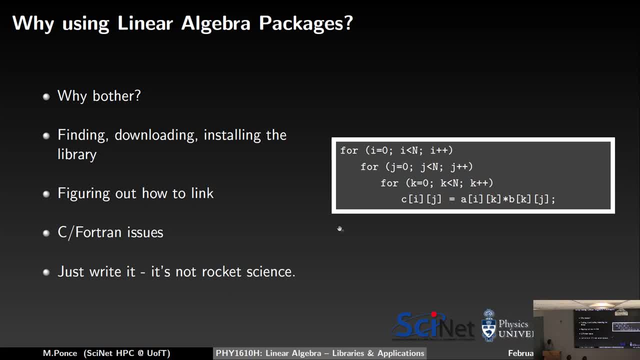 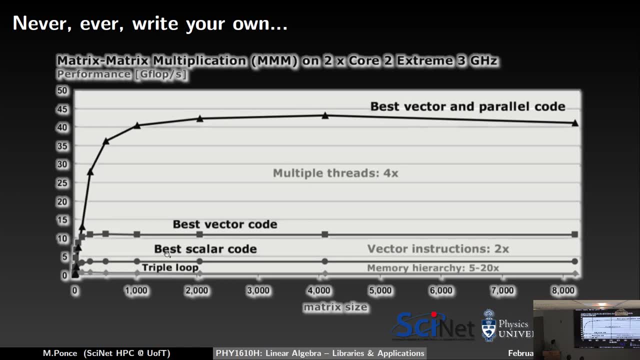 So the triple loop, which was what we were seeing before here, this kind of implementation gives you this number of operations per second. You can easily achieve a factor of two if you use vector instructions. We haven't talked much about vector instructions, have we? 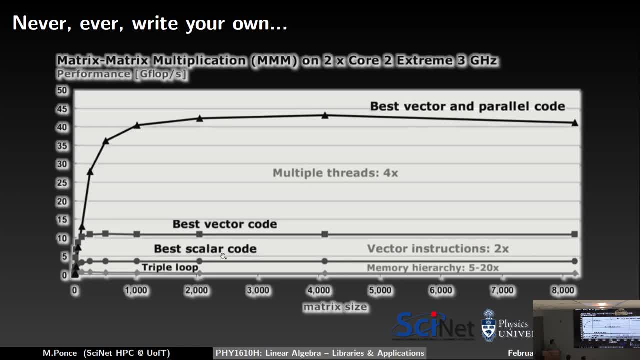 I don't think so. So vector instruction is something quite interesting And it's very useful. It's something that is available to use in modern chips, in modern CPUs, And this that is: you have a vector the compiler can figure out: okay, this is a vector, and 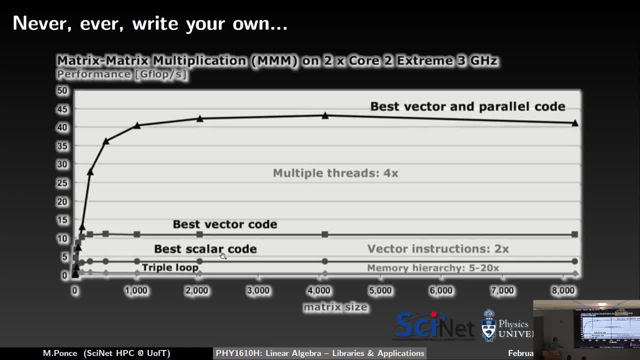 you can have to do operations like adding two vectors. It can add all of them together at the same time, So some of these libraries may take that into account. So then you can have multithreads, like using more than one thing, one core per node, like in the case of Signet. you have been using Signet, you know that. 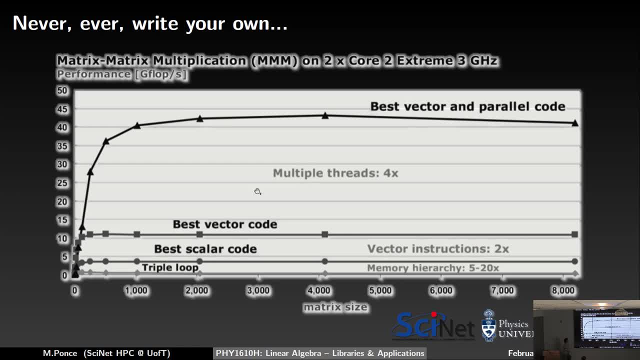 there are eight cores in each node, so you can have multi-threads or you can have even the best implementation: vector and parallel codes working together and you can see that the performance is quite remarkable. So, implementing, closing this gap between the vector and parallel code and the triple 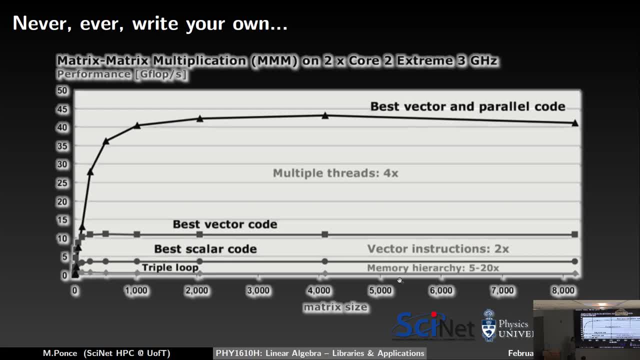 loop that one can naively try to implement is not easy to achieve and some of these libraries, especially the parallel versions of these libraries, do a great job, getting the best performance that you can achieve on top of being pruned of bugs that have been. 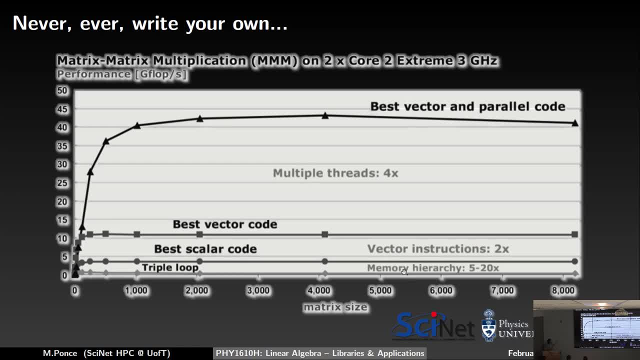 tested for a while, So I hope that this kind of convinces you. why going through the pain of learning the cryptic names and using those libraries instead of implementing your own? Okay, Any questions? The matrix size: is it going to be an n by n or just n? 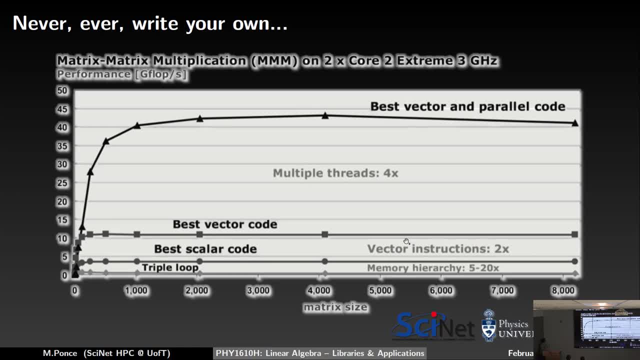 What do you mean n by n? Oh, in this case, Yeah, Yes, in this case it may be. I don't know if we have information about that in the plot, but let's take the simplest case as an n-squared matrix, and then yeah, on top. 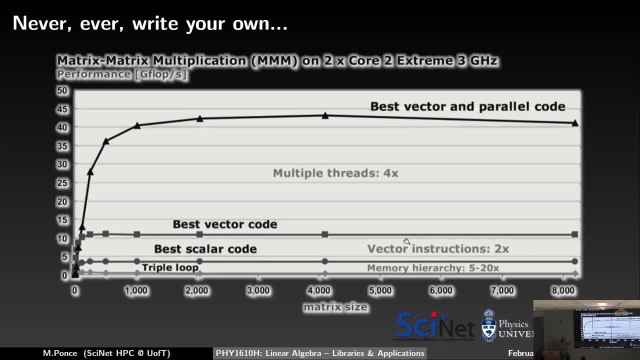 of that. you can have routines like saying: okay, if it is a banded matrix, it's going to be an n-squared matrix. That makes things even better, right, Because I know about the structure and I can take advantage of that. 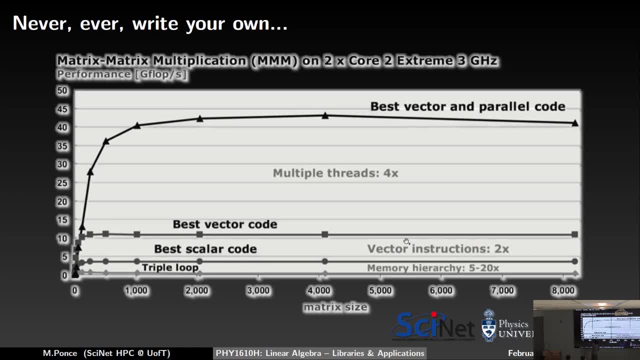 I didn't talk much, but there is also- I don't think there is- information here, but there is also memory issues, right, And we're going to see we have been discussing since the PDE class that some matrices may have this special structure like banded matrices, right. 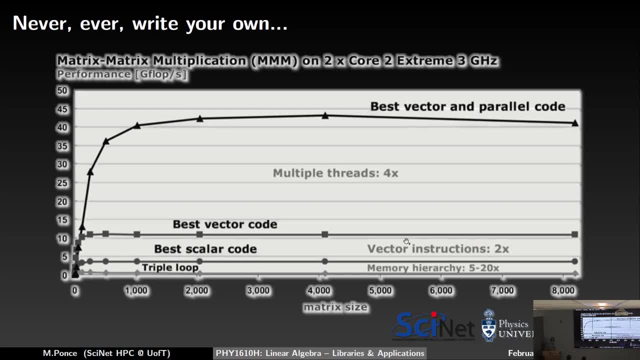 And if I'm dealing with a stencil that has, I don't know, 10,000 by 10,000, I don't know, I don't need to do that. Okay, I don't need to store 10,000 square elements for that matrix. 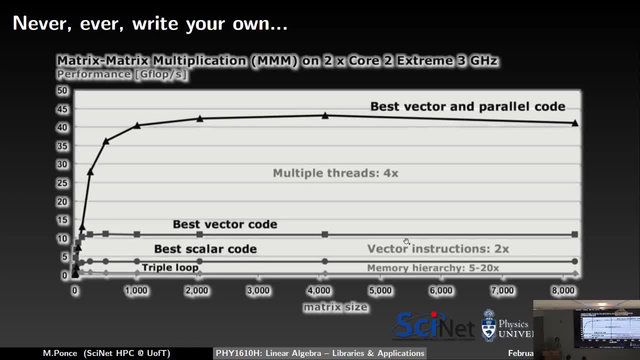 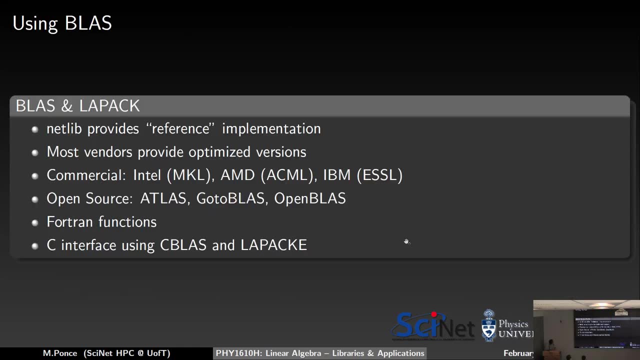 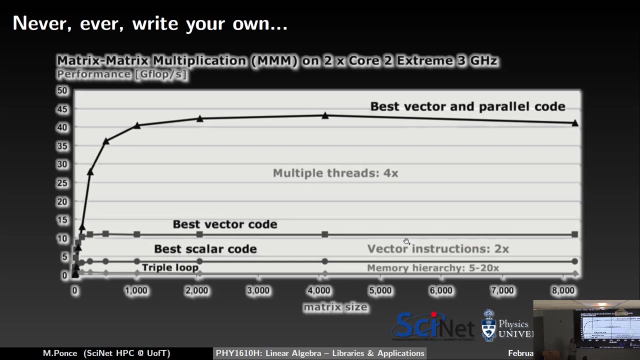 I can just store the diagonal, upper and lower diagonals, right, But I can take advantage of that at the moment of implementing my multiplication routines, right, And Blas knows about that. Okay, Yep, Sorry, The y-axis is basically the performance of the routine. 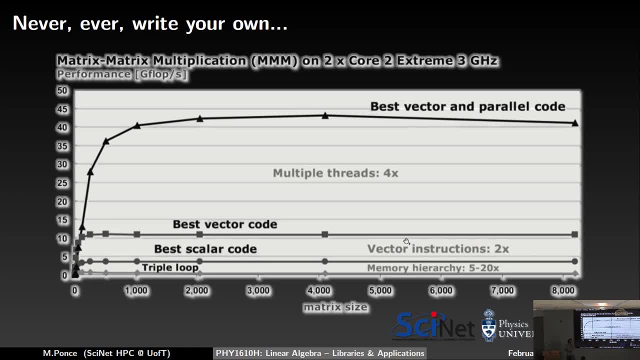 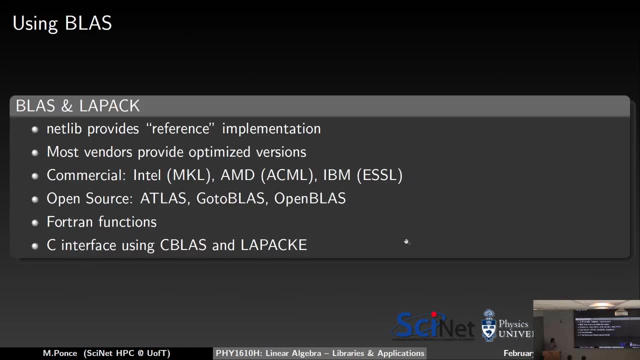 So the y-axis is better performance. You get more floating point operations per second, And I think about Any other questions. Okay, So let's go back to Blas and LIPACK. So these are references are provided by the NetLib implementation. 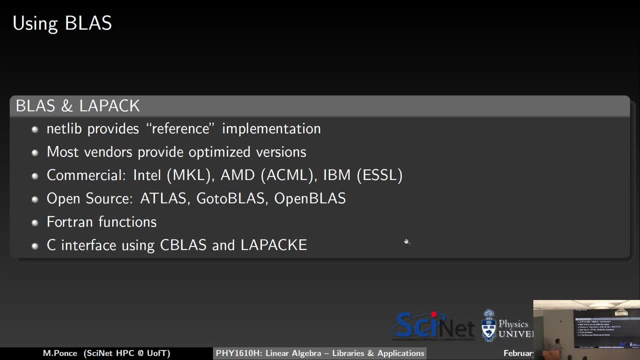 I think I have a link. I'll link at the beginning. The thing is that many vendors or commercial software provide their own versions specialized for their own hardware, for instance, like Intel has MKL. So it's as good, or in some cases even better, than these ones. 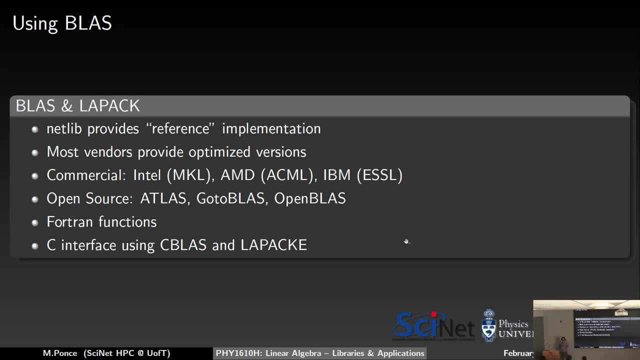 AMD provides HTML And then IBM has ESSL. Open source variants of those are Aclas. Go to Blas, Open Blas. Open Blas is quite neat because it's pretty easy to install and follow. So I have an example, using actually Open Blas, I think. 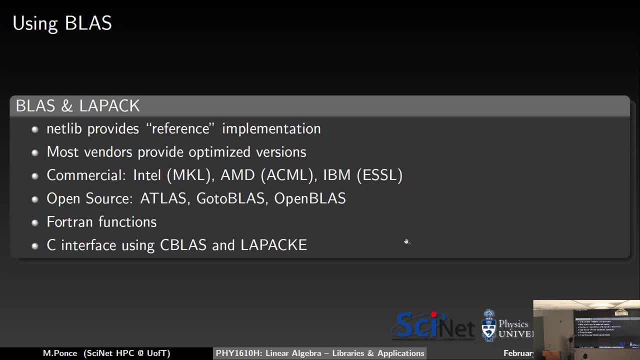 As I said, there are many Fortran functions, but there are also C interfaces using C Blas and LIPACK. So I have an example to show the difference when you are calling one of the Fortran functions, the Fortran calls and the C call. 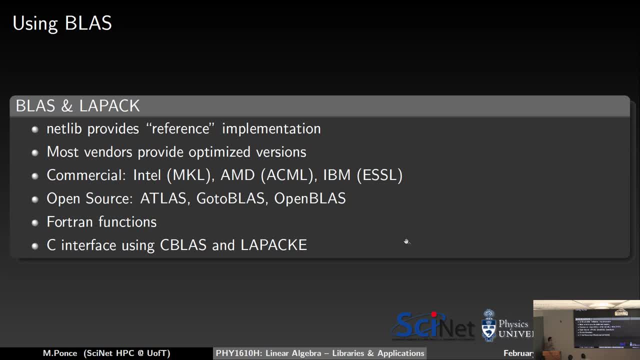 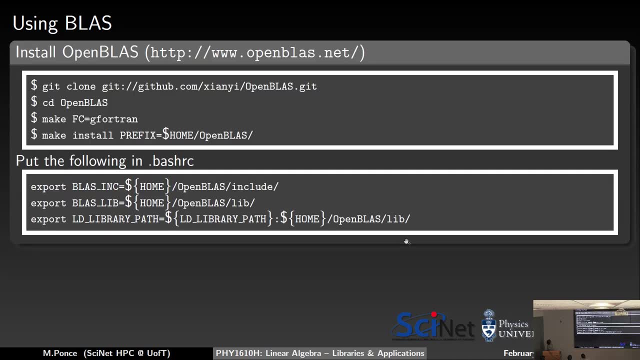 And the main difference is how the different language deal with passing around. It's passing arrays or not. That's the main difference. So how to install Blas, How to use Blas, So let's say this first part. if you want to install in your own computer, this is one. 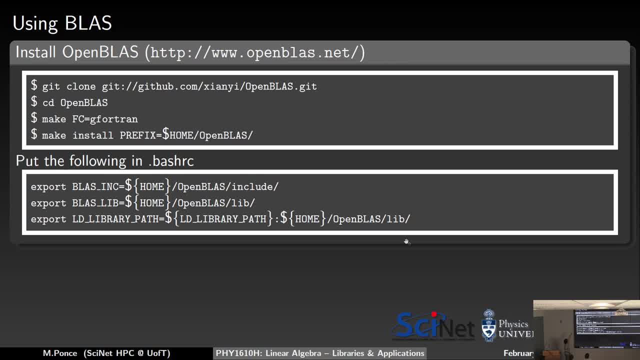 of the easiest libraries to install. So basically you can clone this GitHub repository for Open Blas. Just clone that repository, Go to the Open Blas directory, Choose. You will have to have a Fortran compiler. I told you these are Fortran routines, so you will have to have a Fortran compiler, like. 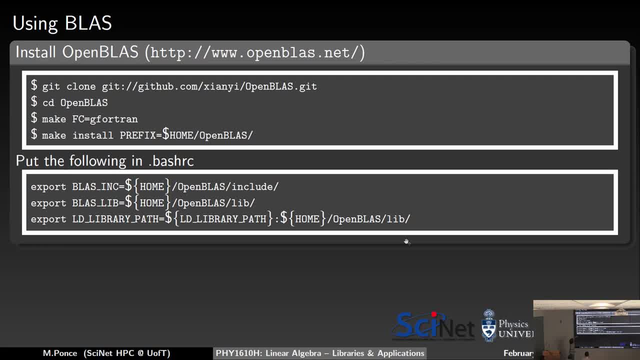 gFortran. for instance, Do a make for preparing the installation like it's going to compile the routines. when you do make, And by setting FC equals gFortran. basically, you are telling the main file to set the variable of the Fortran compiler to gFortran. 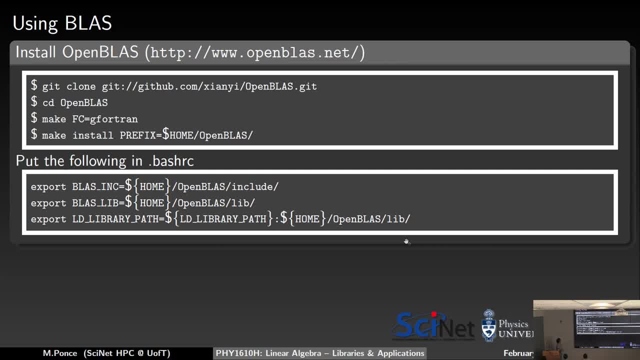 If you have another Fortran compiler, choose your favorite one. If you leave it without specifying, I think it will try to figure out which Fortran compiler this is. It will try to figure out which one is installing your system And then for installing, just to make install and set the prefix to whatever you want to. 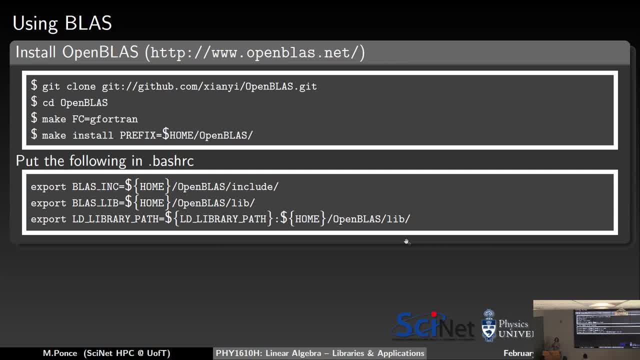 install, For instance, your home directory and then Open Blas whatever you want. Okay, Just remember that you will need to know where the installation is going to happen, where you want to install the libraries. Okay For linking. so this is the installation part. 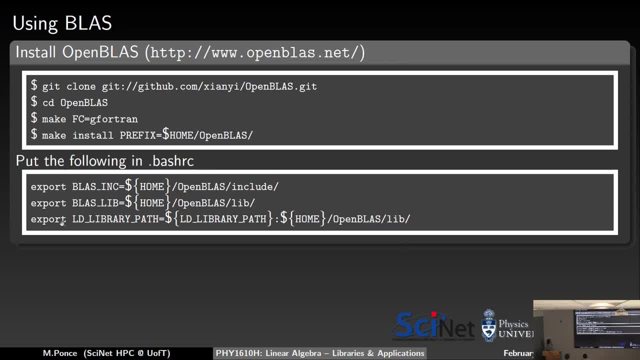 First part is just installation. The second part is a suggestion How to make the header and library directories available for you always when you want to compile your code. So in this case, one suggestion is: go to your bashrc file. that is loaded every time. 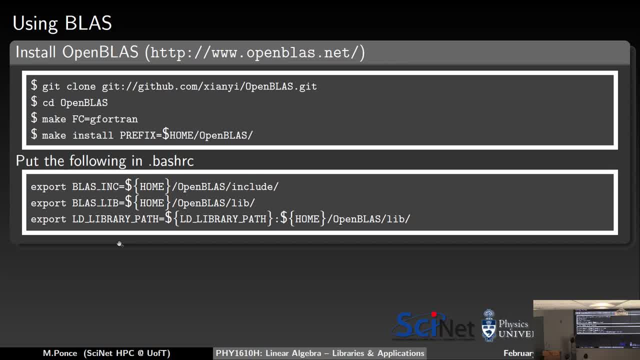 you open a session in your terminal And add this slice So Sport Blas Inc. That's the header directory And then, wherever you put it, it will be an include directory with the header functions as we defined When we. when RAS is so, discusses modularity. 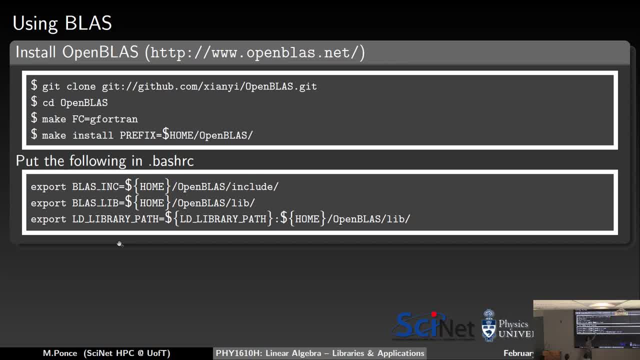 And then there is another directory, lib, where the actual libraries are going to be, So that's, you can name it BlasLib. Those are suggested names. You can use the names that you want. And finally, because these are libraries that are dynamically linked, when you compile set. 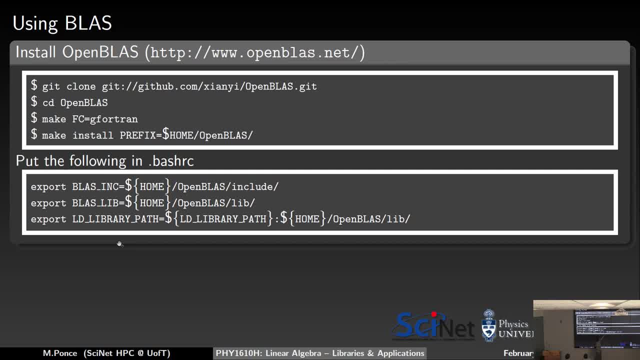 the LD library path to whatever was before, plus the new directory where you installed the libraries of Open Blas. Okay, Yep, Here Whatever was before in your system. So if you have other libraries that you have installed before, LD library path will. 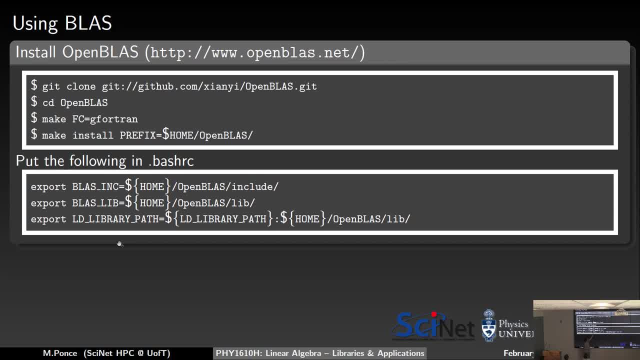 have that for sure. If it is empty, it's empty, And this may be the first one. By the end of the course you probably will have this. You will have next-cdf gsl- Another one I'm forgetting. 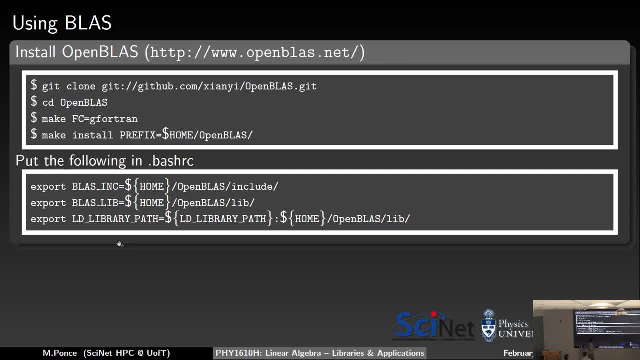 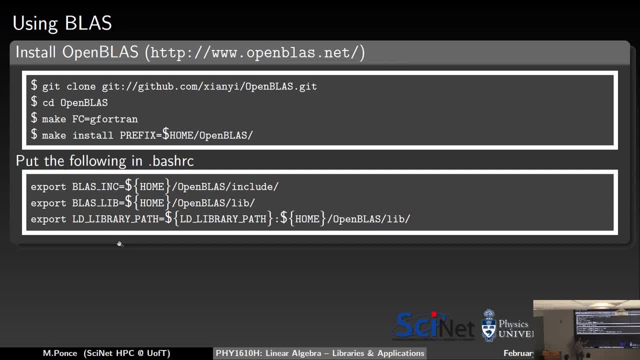 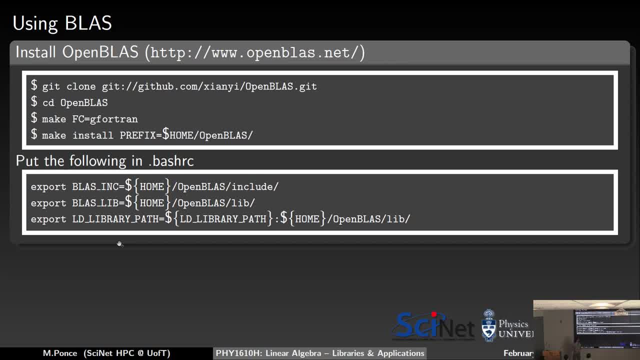 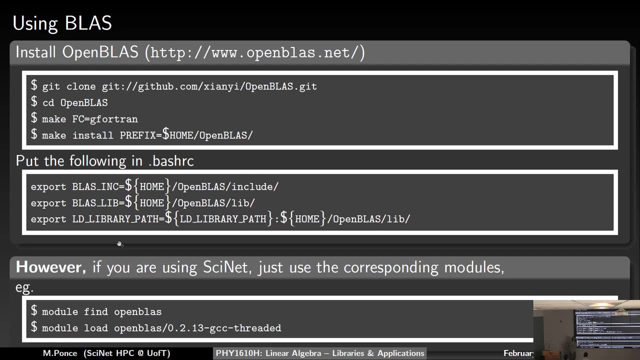 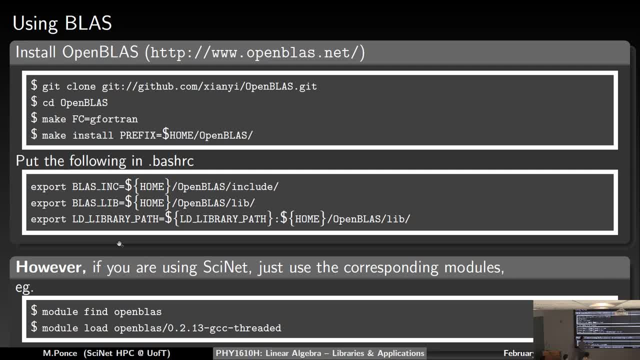 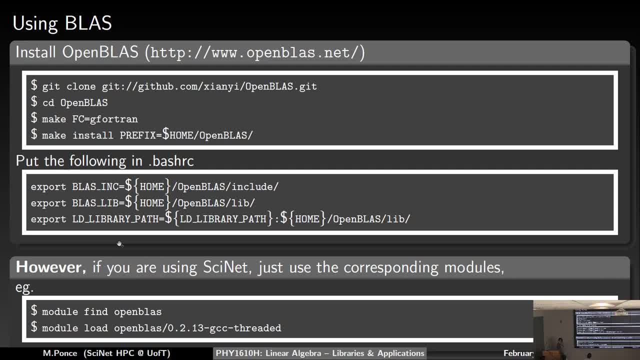 Okay, Okay, Okay, Okay. Any questions about this? The installation should go pretty smooth. It's not one of these libraries that give you headaches when you're installing. even on Mac OS, I think it works just fine. Okay, So let's take a look at one simple. 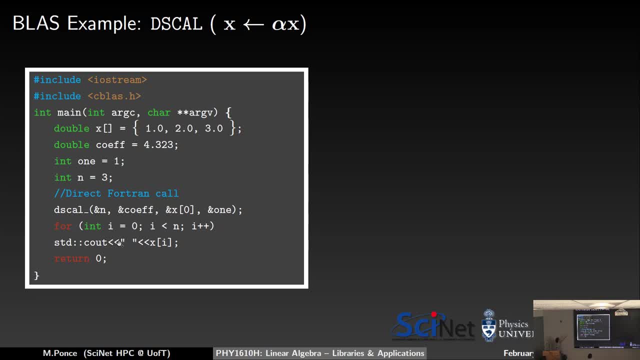 example. So we're going to start easy. So this is just a scalar vector multiplication And one of the things that you will see is that this routine starts to recycle a lot. You are kind of eco-friendly to eco-friendly, if you ask. What I mean with that is that if you have a vector X and you want to, 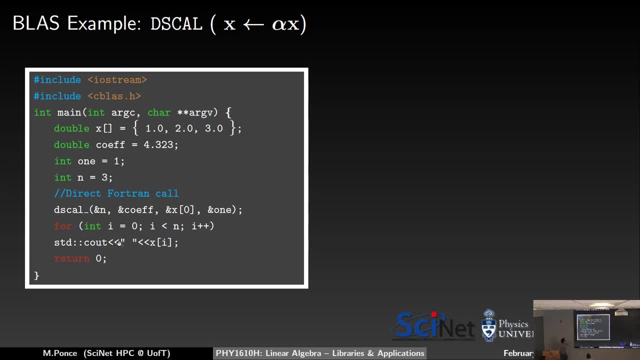 multiply or scale the vector. that's how they call it. a scale the vector by a coefficient. it's going to store the result in the same vector that you use. Okay, So let's take a look at the code. So we are doing, including the usual. 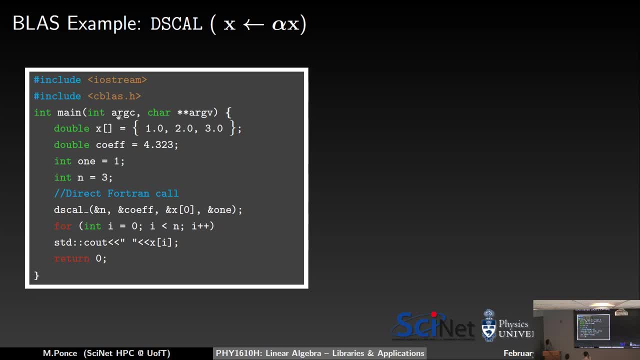 library iString. So we are doing including the usual library iString. So we are doing including the usual library iString. and now we are going: this is the new library cblast, the header file, the arguments, as usual. so here we have a vector 1, 2, 3, the coefficient that we 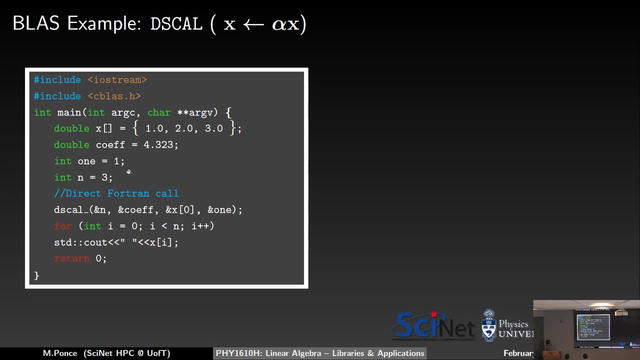 want to use for multiply, this guy will. I will explain a second. so basically this routine allow you to do the multiplication and take like strides. so if I want to multiply only the first, third and fifth element of the vector, I can say 2 so it will jump. so it's a strike in the elements of the big. so in 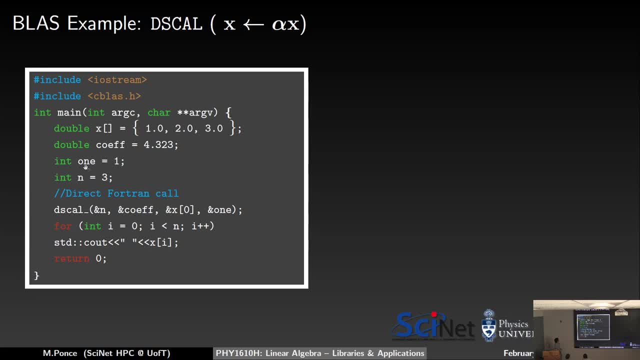 this case I want to multiply all the elements of Asia's. you need to specify the size of the vector and 3, and in this case I'm having just a direct for tranquil. so is the sky. so it's a double type of vector: is a scalar or a scale in? 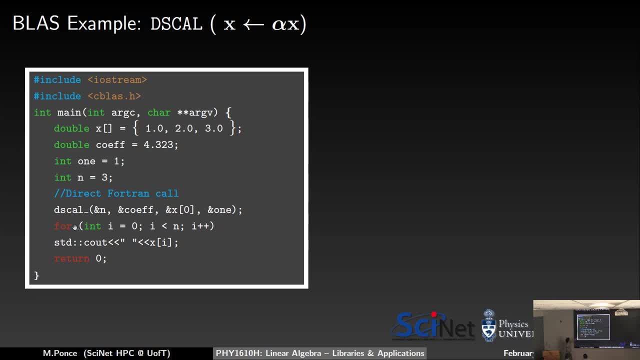 the vector or a scalar multiplication of the vector, and you notice that the fourth one call has an underscore. the other thing that you will notice is I'm passing the content of the variables, and this is because the way that Fortran passes the variables- okay, it's different. 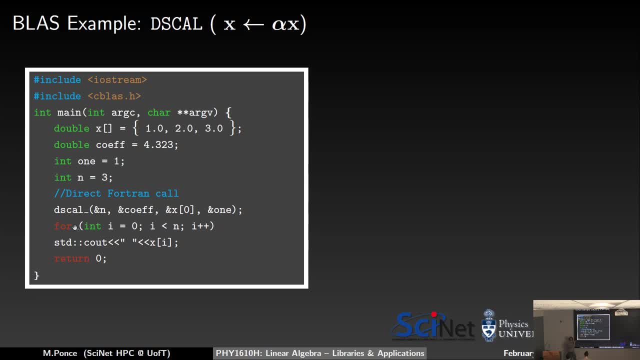 than from C that pass for by reference. in the case of Fortran, pass by value. okay now, because we want the result- and I told you the result is a store in the vector itself- we had to pass by by value, but the first element, so we know where. 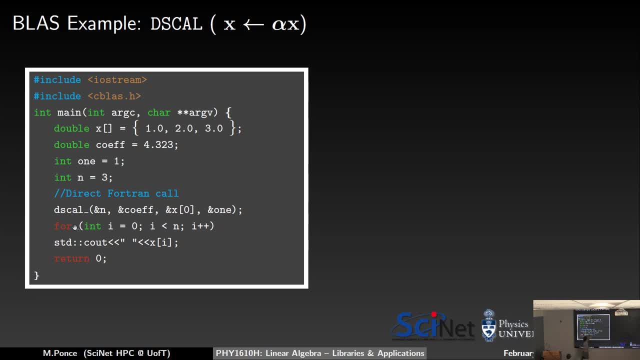 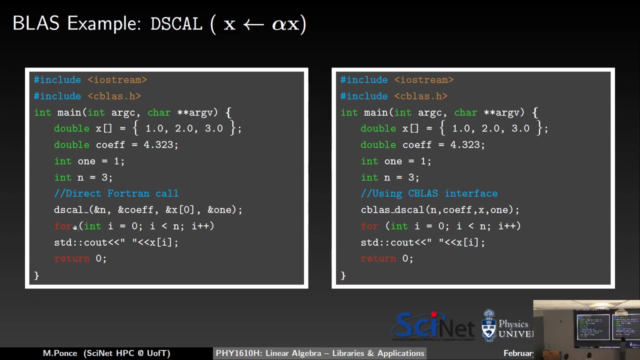 to put the data back, so that's why we're doing this. basically, this for loop is just for printing the result, but before showing how it looks, how, what, what it prints out, let me show you the C version. so, in this case, while using the, the C blast. 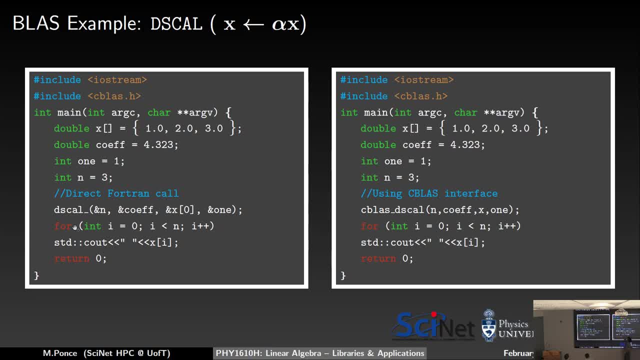 implementation or interface. so in this case you need to add a C blast underscore thin before the name of the function. it's the same function. d is called, but in this case is C blast and you can notice. you don't need to pass anything by by value itself, you just go as the pointer in C and the 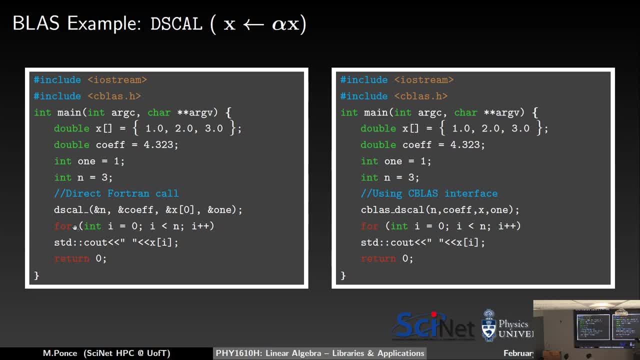 rest of the code is exactly the same. okay, any questions about this. they are not being used, but is issue, which is good practice in case. that your code, but you can leave it void if you want similar with the returns here. we talk about that before how to compile. okay, 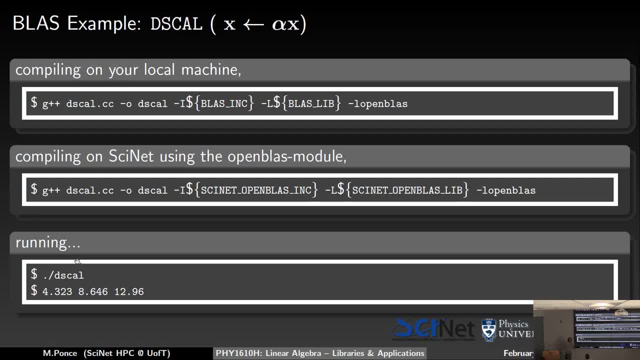 let's say that we want to compile on your local machine. remember, we feel we put the values of the installation path in this variable- blast inc and blast leap- and basically I'm using the C++ compiler. the name of the code is dsqlccc. want to generate the, the file called the dsql I had to include, remember. 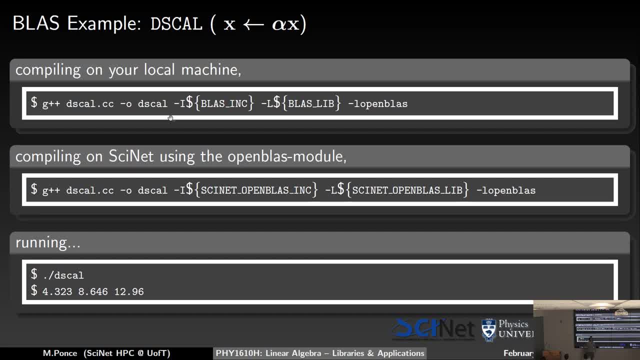 But this, minus capital. I is where the header files of the functions I want to use are. So in this case are the header files of the cblast implementation or the Fortran implementation, but whatever those are, are in the blastinc directory that we defined before. 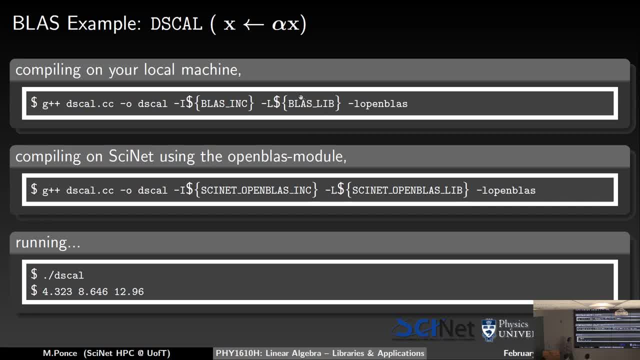 I need to include also where the library files are. thus we do with minus capital L. And finally, we need a flag for saying that we want to use the open blast library. So this is the last flag, this tiny L: open blast here. 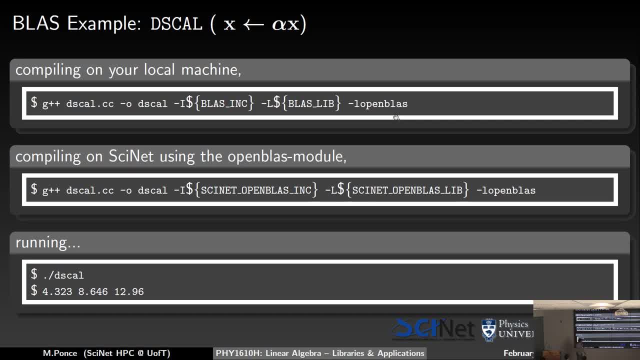 Yeah, you do. minus I whatever header file. minus I whatever header file. If you are using signet, this is the nomenclature I was mentioning. you will notice all the modules have this nomenclature: signet. underscore the name of the module, underscore inc. and. 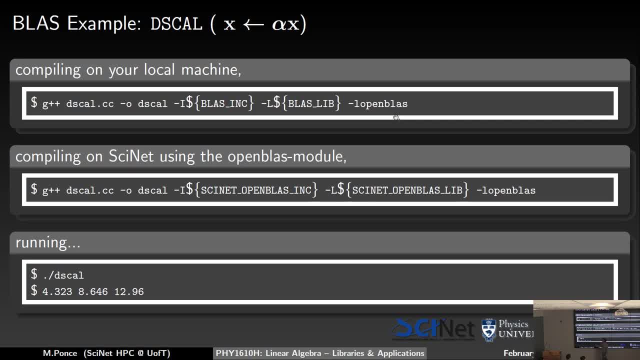 the same for the library signet: underscore The name of the module, open blast, in this case underscore lib. Okay, So that is the advantage of doing things on signet. You don't need to install anything, just load the appropriate module and then use those. 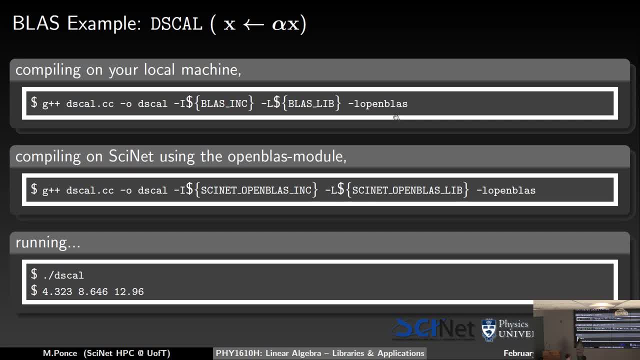 those genetic variables? Yeah, When you say confiling on signet, do you mean like when, for example, in the future, we are going to use the signet thing or something? is that what you mean? Or now, I know that some of you- at least one of you- was using signet for solving the modularization. 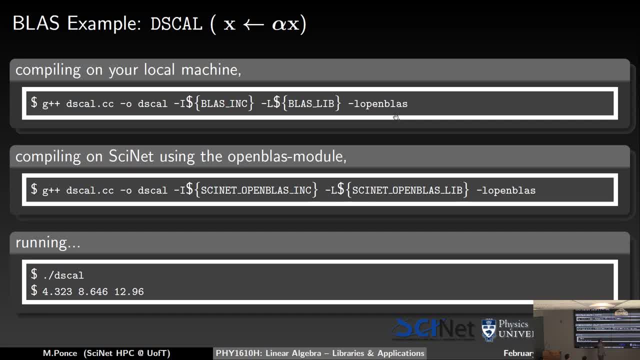 assignment. I think Okay, So you are welcome to try and use signet from now on if you want. Okay, I have no idea, Unless that we ask you to install a particular library in one assignment, but I don't think. 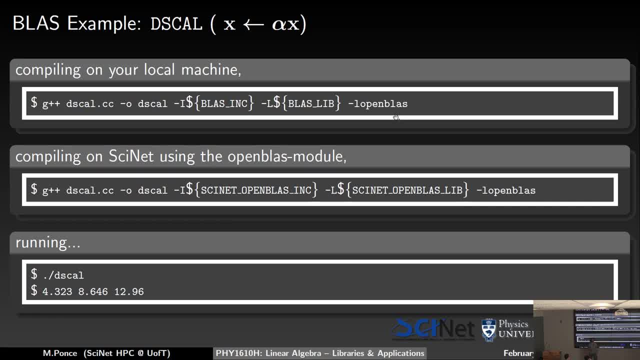 that's the case. Even RRA is installed on signet. so, yeah, If you feel like, okay, I want to compile things on signet. don't screw my machine or whatever you can do it, Just use the libraries that we have installed on signet. 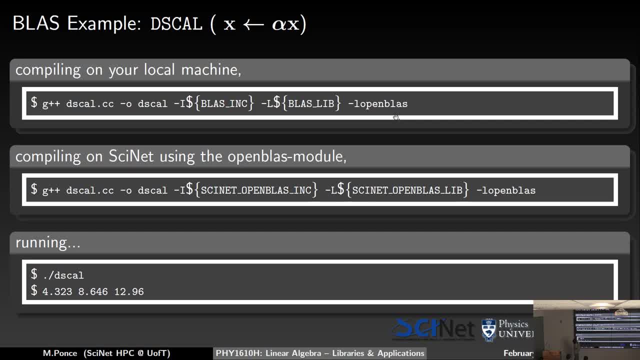 Okay, You won't see. let me see so far, until no. next week. the next week, Okay. Until the next one or two weeks from now. probably you won't see any difference in the codes because they are not too compute intense. but yeah, you can try and use signet, right? 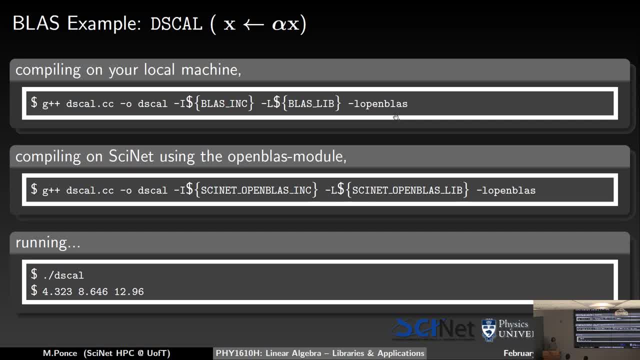 now. Actually, it's a good practice because we will know if your accounts are working or not. I think all of them will be working, because if you can log in with your signet credentials into the education website, it should be working. but it's not a bad idea to start trying. 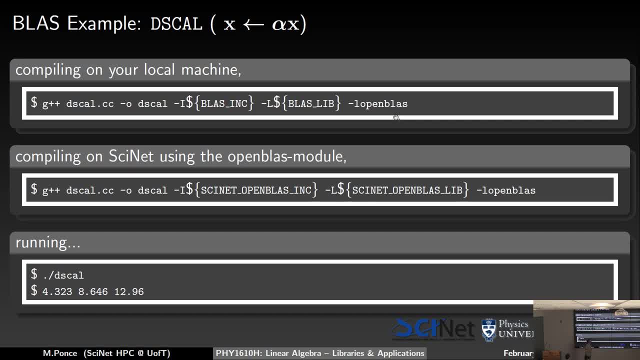 I just wanted to explain this, however, in the course, because I actually have no idea how to actually use signet. Okay, Okay, So my first suggestion is: we have, on March 8th, an intro to signet and we may have a. 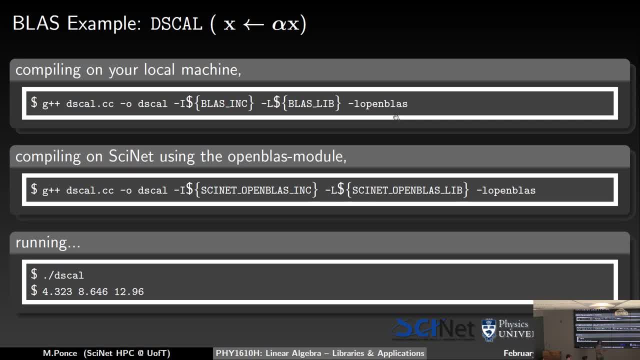 mini intro to signet in one of these lectures. But yeah, so if you don't know how to just use your computer, it's just in case that I know some of you may be using and also it's a good idea just to mention that these 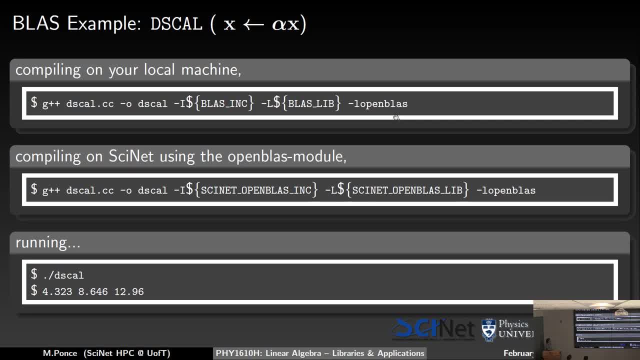 things are available on signet. Okay, So this is compilation. We have just one module or one file, so we don't need to worry much about linking with other modules. But remember you will need to include these guys- the header and the library path, in order. 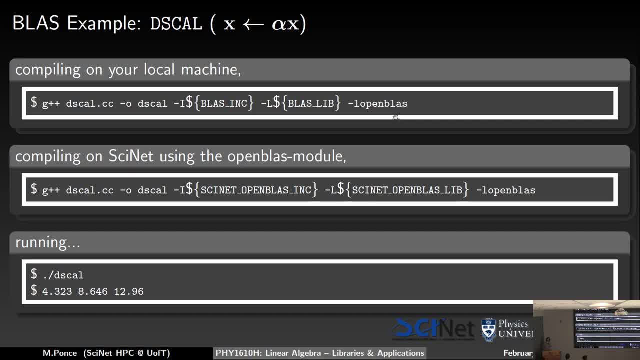 to the compiler for finding the appropriate routines that you want to use in the implementation. How to run it? Pretty easy, Just the name of the thing and it runs. And basically because I was printing the elements of the array, it's just printing. 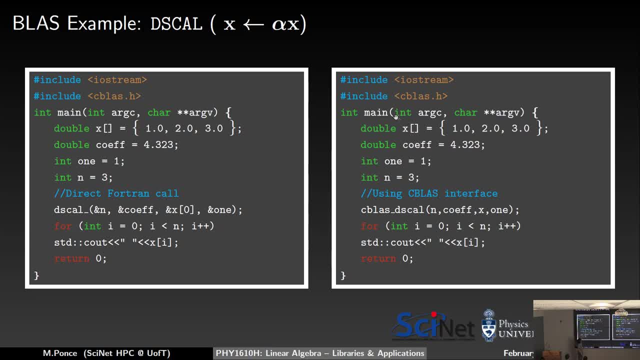 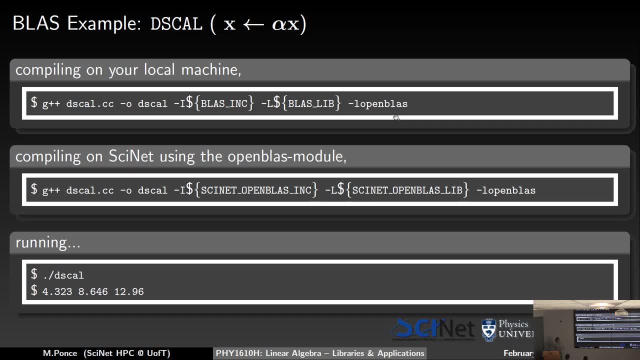 the Scaled version, so that number 4323 multiplied by each of those numbers and that is what it's printing out. Okay, So it looks like a lot of trouble, like remembering compilation flags, remembering the cryptic names of the routines, just for doing a multiplication of elements, but things 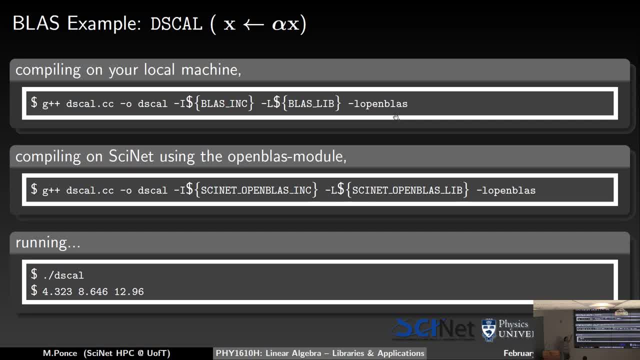 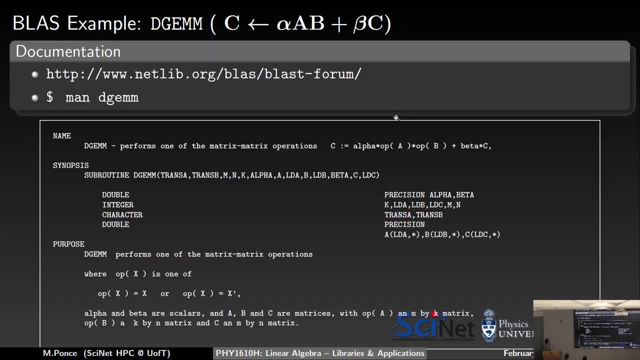 are going to scale up to be more interesting and more complicated, and this is how we start. Okay, Any questions? No, Okay, So I tell you, many of these things are kind of cryptic, at least in the name part. 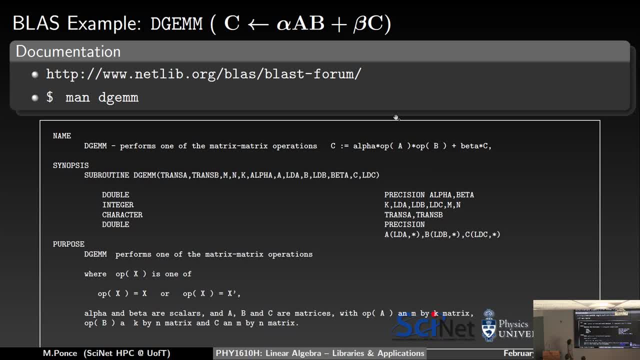 You can find a lot of help. in particular is the Netlib reference guy, if you wish, And also the funny thing or the nice thing that happens with these libraries is when you install it, it also installs in a man file for you. 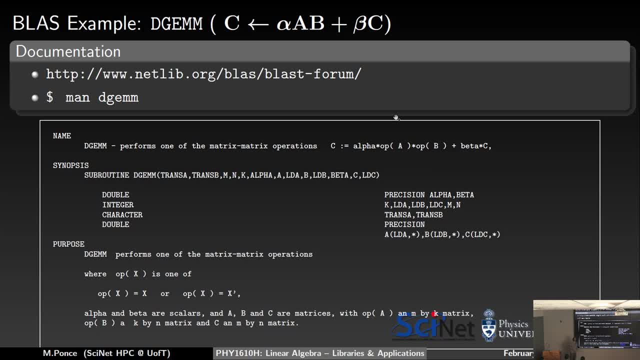 So man files are help files that you can use with the man command, which stands for manual. So if I don't exactly know how to use the double general matrix, matrix multiplication, that's TCEMM, I can do just man TCEMM, wherever the library is installed. 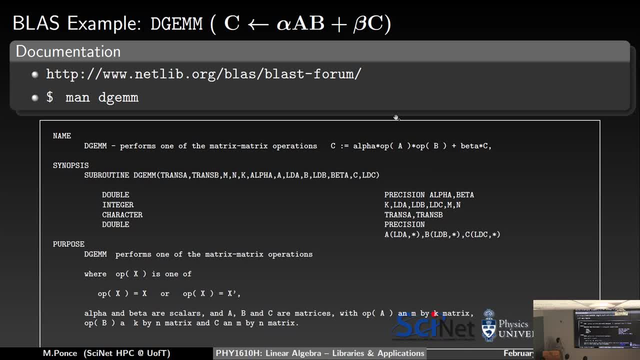 And then it will pop up a help page saying: okay, this performs one of the matrix matrix operations. And basically the way to say is, when you do one matrix matrix operation, always think that these things do more than one thing. So it can also do the matrix A multiplied by the matrix B, but also multiplied by a. 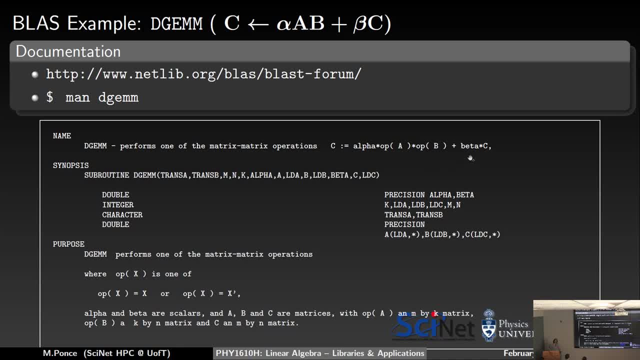 coefficient Another. It can also do the matrix multiply by another term. So that's the matrix matrix version. It tells you basically what type has to be each of the parameters that you are going to use in the function and it also tells you a bit of the help, a bit of what these 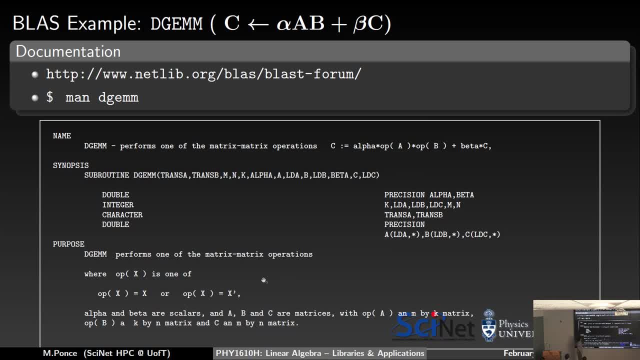 things are. So in this case, operator X and operator X prime, and the matrices A and B and the dimensions, And this page continues. So there are several lines of help there. Okay, Yes, So far we haven't done anything at all related to parallelization and these versions, the 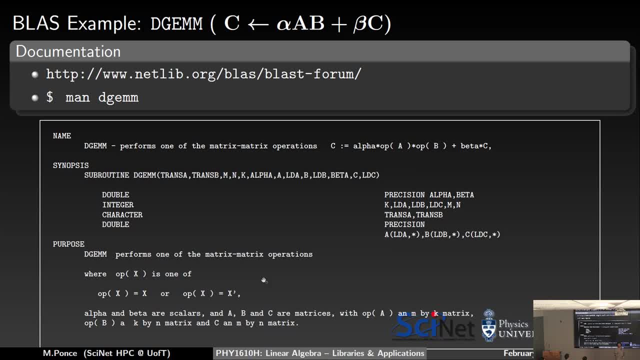 versions that we're discussing today: BLAST, CBLAST, LAPACK or LAPACK-E. don't do parallelization for you. There are parallel versions. ScalaPack is the one for LAPACK, I think Remember Probably Yes. 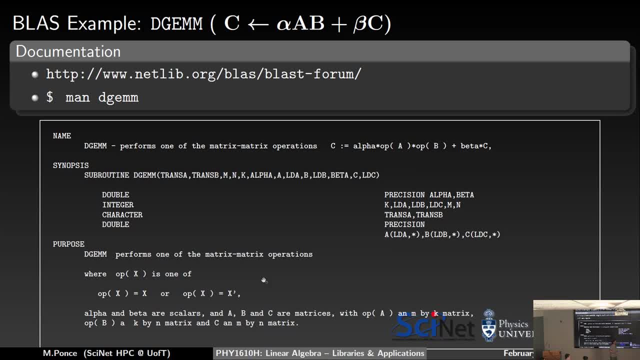 It's a credit, So on a note, part of BLAST. So just using the course on the note the library can do it, Not the reference one, But OpenBLAST or MLSTL for you if you take the library version as parallelization. 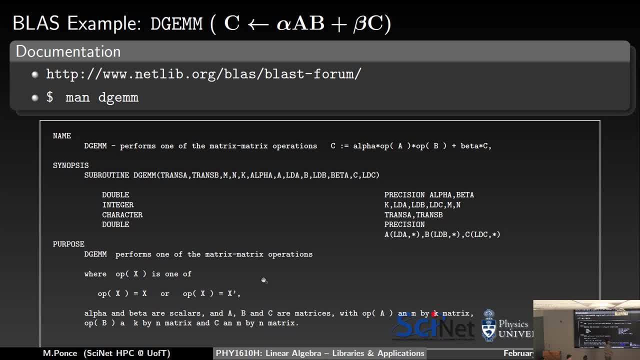 But if we take the full time, same speed as No, No, no, no, no, It's not the same, It's more like a Because it doesn't do, because it has never thing, Yeah, Yeah. 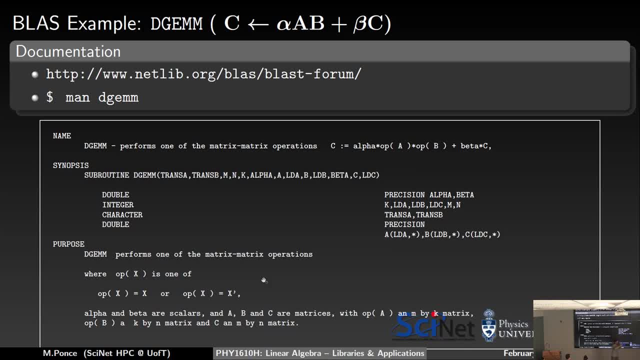 Yeah, It doesn't do that simple and naive approach of the three nested loops. That's something. I don't even know what it does, but that's something that's. That's an advanced class, Yeah, That we had to take. 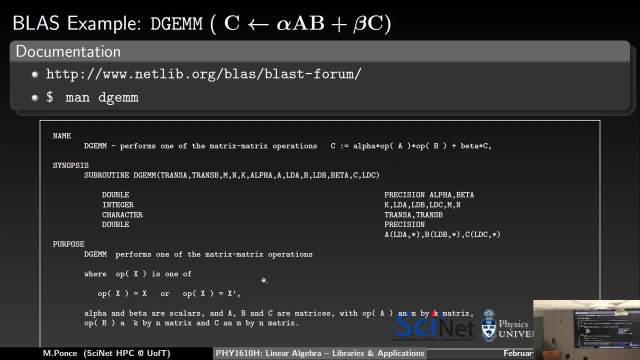 But you don't have to take The library, is there? Yeah, It's like All right, What else going to start to see something funny? so, as you can see, so this is a matrix, matrix, multiplication, and you see at the arguments there are like how many one. 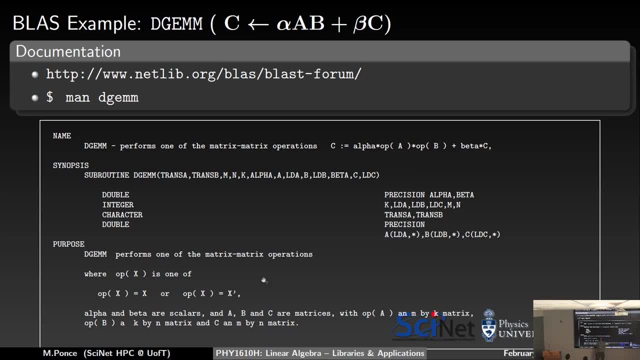 two, three, four, five, six, seven, eight, nine, ten like more than ten arguments there. so I told you it's actually doing just not matrix, matrix multiplication. it has the the possibility of computing a scalar in front of the matrix matrix multiplication, adding another term. but it also has the chance of specifying. 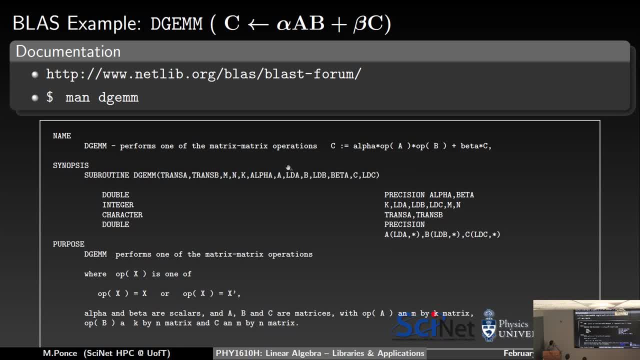 something underlying the structure of the matrix, and these things are this: LDA, ldb and ldc indicators, which stands for leading dimension of the matrix, a matrix, B matrices. so what we mean with that is you can actually take a matrix, and for whatever reason, one to multiply three times one. you can actually take a matrix, and for whatever reason, one to 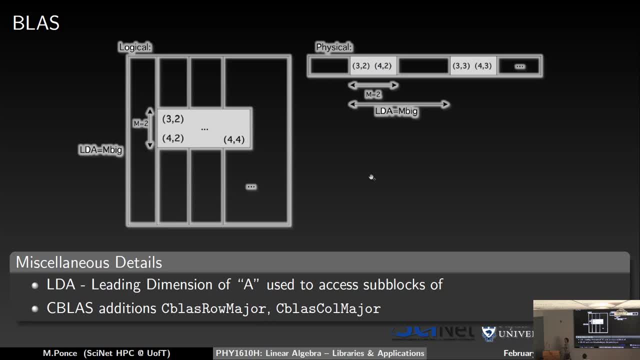 multiply three times one, you can actually take a matrix and, for whatever reason, sub-blocks of the matrices and not the whole matrix per se. if you want kind of an artificial example of how this work, think about this canonical sort of the composition that we told last class, where the matrix not necessarily has to. 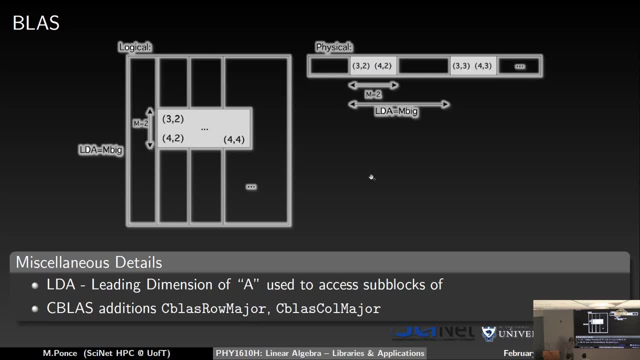 be diagonalized, but it can be diagonalized by blocks, depending on the, on the nature of the matrix. the point being is you can specify the blocks that you want to take in the matrix to do the operation alone and not the whole matrix. and how you do that, you do with this leading dimension of the matrix. so 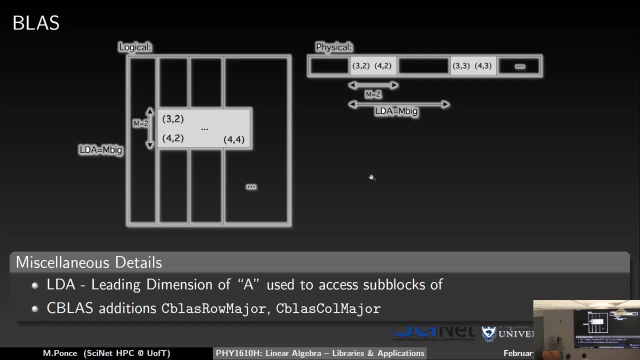 logically, your matrix, or you may think of your matrix like this rectangular thing we talk about, the. how we store the things on memory physically is an allocation of consecutive spaces in memory. hopefully, and these let's say that you want to just consider this sub block in the matrix. so we had the. 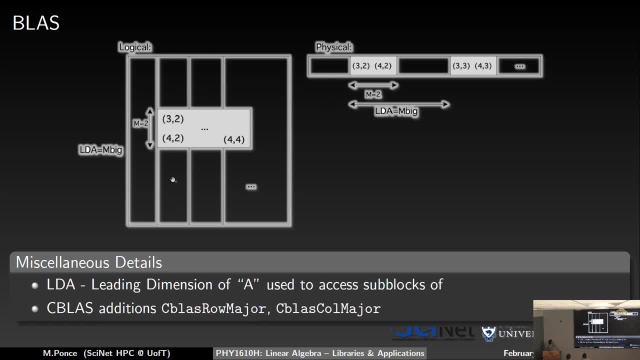 element three, two and four, two, because this is row may your store. you Will be consecutive: the first element in the row and this, and then the second, and then will come Because it's a store. then you have a gap until the next part of the block Okay, which it will be the element for. 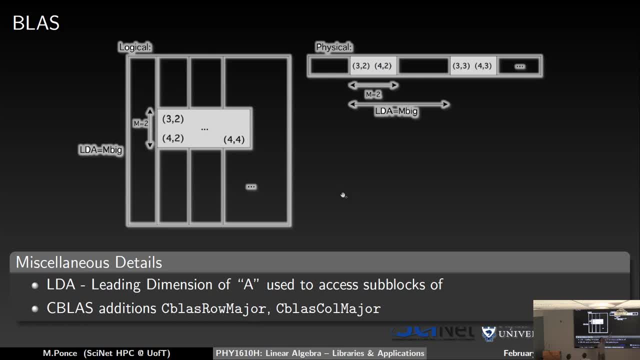 Three, three and four, three. right, those are the next. one day Now, if I want to do that, if I want to consider these two blocks, I had to specify which is the leading dimension, Which is the shamp that I have to have there in order to reach the next. 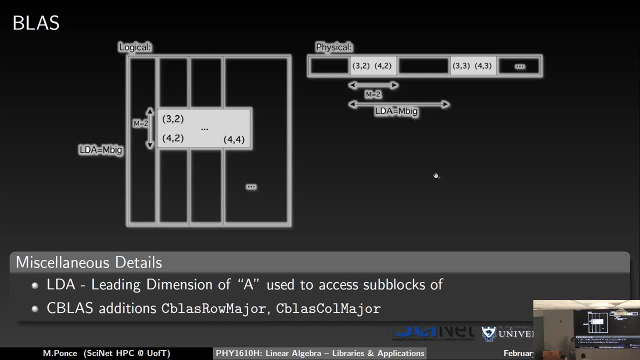 Okay, usually you won't do that, but this a feature the routine have for you. Okay, in general you put just that equal to the dimension of the matrix, like an m by m matrix, and you are done. But in case that you may consider, you may want to specify something else there. 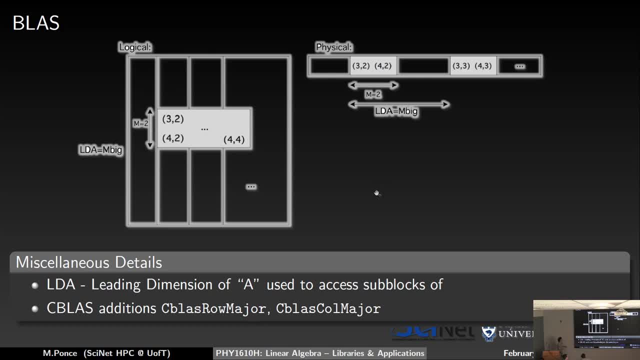 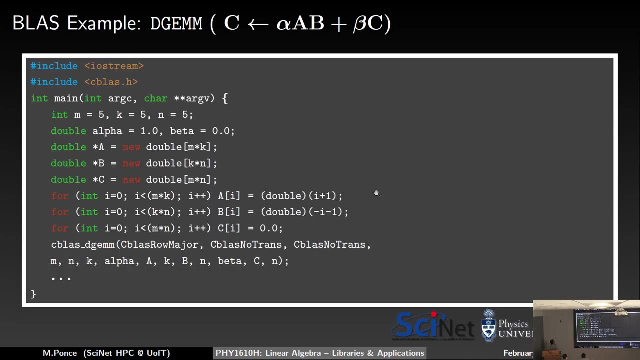 Okay, In addition to that, the C blast also allow you to store things at your own way, like having row major or column major implementations of the matrix, How you, how you lay down the matrix in them. So let's take a look at how we actually implement this. and the other thing is- I told you this at the beginning- all this, 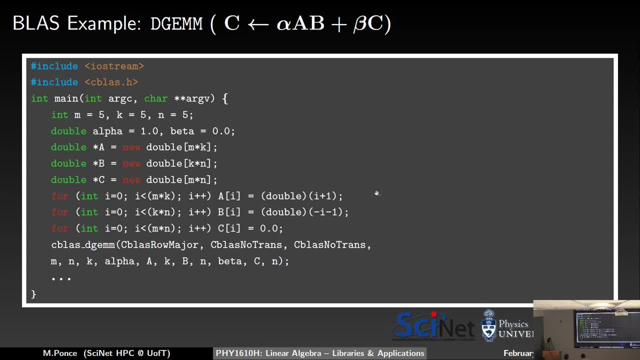 Recycle. things keep coming along. So if I want to store the, if I want to actually perform the whole operation of alpha times a, times B Plus beta times C, all is going to be a store in C. If you don't have a third matrix, this is where actually your result of the matrix multiplication going to be. 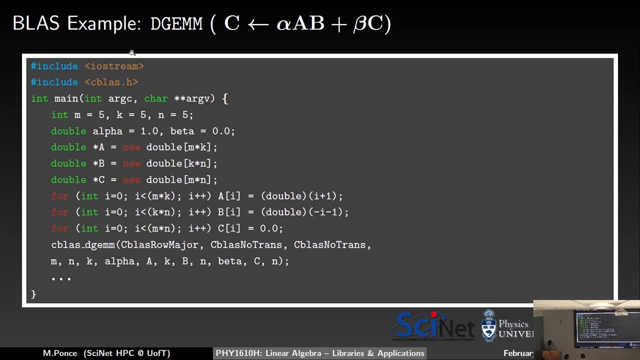 Okay. So again this is an example of the double shadow matrix matrix multiplication. We use C, C blast, so in this case we will have Mkl and no, sorry, mk n. Phi, which are the dimensions of the matrices, are going to be M by M, K by K and M by n. 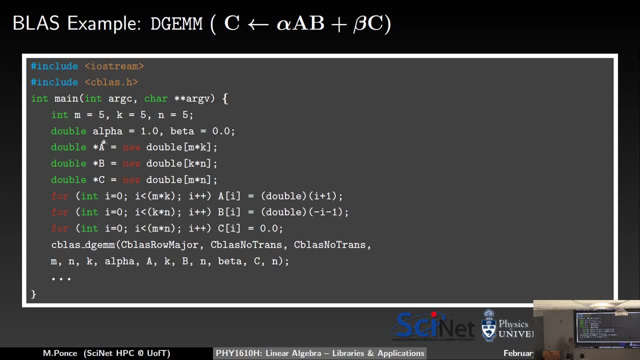 Because we just want to multiply the matrices. alpha is 1, So there's the factor in front of a, B multiplication is just 1 and beta is 0, So there is no Western term. right, that's basically what we are saying. We are allocating dynamically a space for. 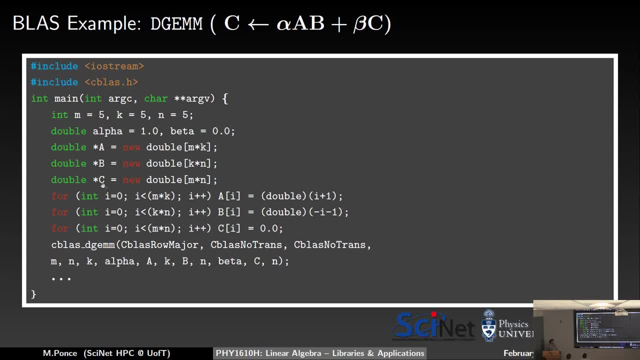 A, B and C. So this is how we actually did deal with two-dimensional arrays or, in this case, matrices, And then we basically just put some values there. So for C, we don't care, it's just a field of zeros. A and B has some given values. 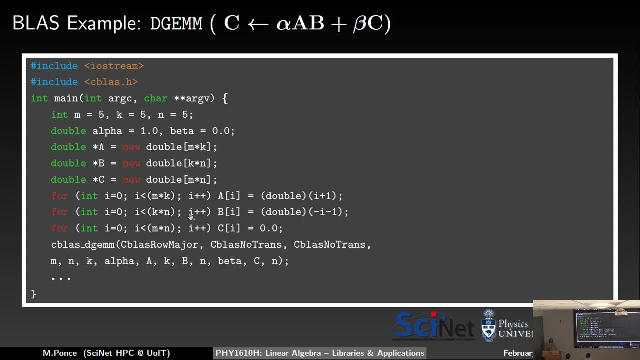 depending on the value of the index that we used to cover. Okay, And the call to the library goes like this: So it's the C implementation. It's the double general matrix-matrix multiplication. We are specifying that we are using row major implementation for putting the data in memory. These are 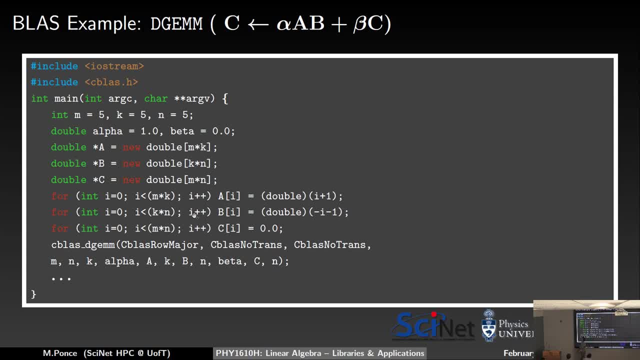 for specifying. You can say: okay, this is the transpose of the matrix or not. So basically, you don't need to transpose, You have the matrix. So in this case, these are not transpose. These are the dimensions of the matrices M and K. The coefficient alpha, which, in this case I say is one, The. 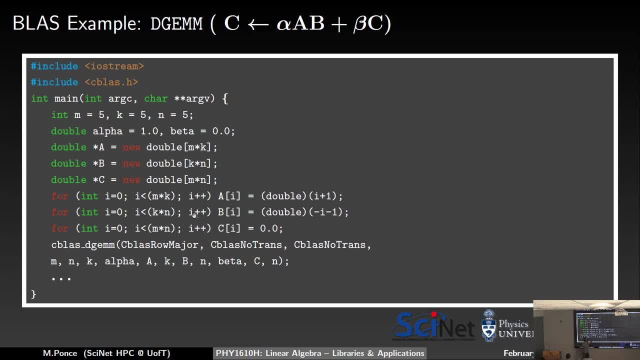 matrix A, The leading dimension of the matrix, because we want the whole matrix- is the same as the dimension of the matrix. The matrix B- The leading dimension of the matrix B- Again because we want the whole matrix- is the dimension of the matrix Beta, which is zero. So even if you don't want, 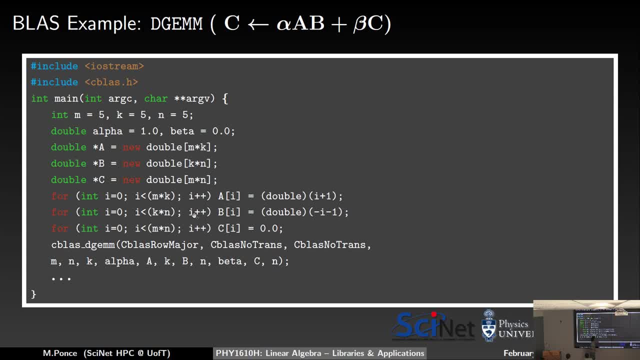 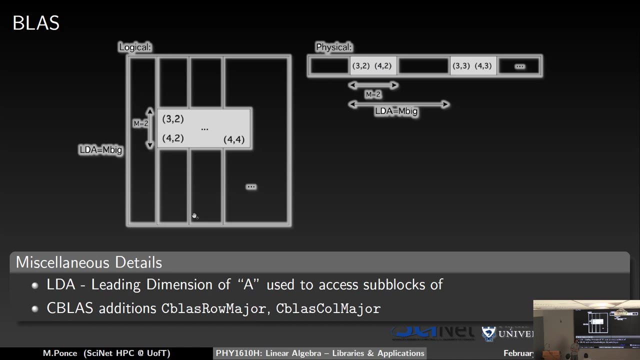 to do the addition with the third matrix, you need to specify that parameter and see what is going to store the result of the matrix multiplication. Okay, These dots are just printing out the matrix. Any questions about this? Yep, So in this case is row major the representation I'm doing in the 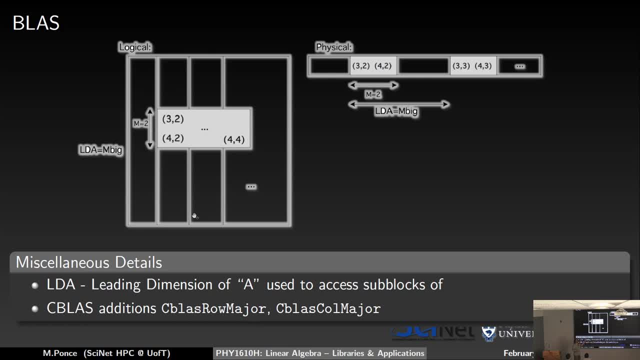 memory layout. But you can specify row major or column major, So it's up to you how you lay down the implementation, the representation of the matrix in the algorithm. You first. Yes, Oh yes, I was saying row major, right, It's column major, Sorry. 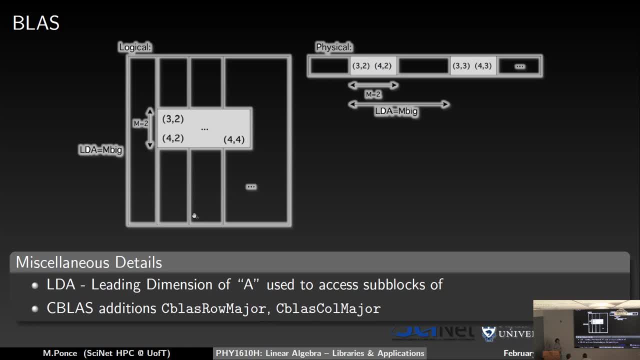 So the picture is called and the reason that it is column major here, because this is talking versus lab. All of this was originally Yeah, So I'm going to do it in four trinameter. So I'm going to do it in four trinameter. 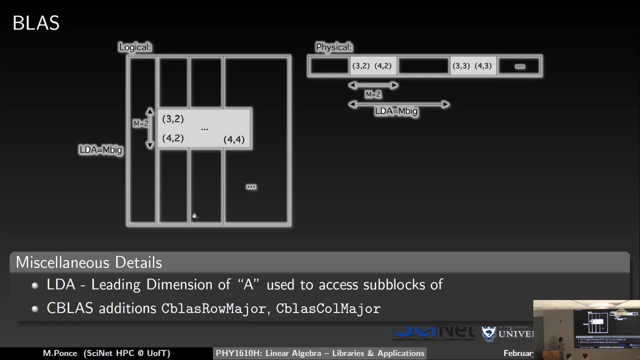 Yeah, So I'm going to do it in four trinameter. So I'm going to do it in four trinameter And you have matrices in both, So let's take a C. We're probably just going to do row major. 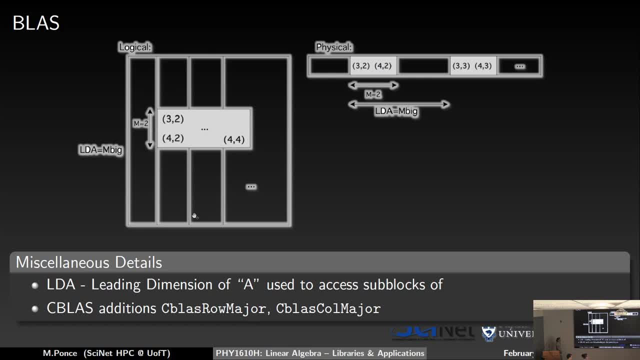 C is very interesting. If you see class is fast, you see class is very good. Row has five packages, like a library of matrices. you can actually pick the way you want. Pick one way and then it will use the time. 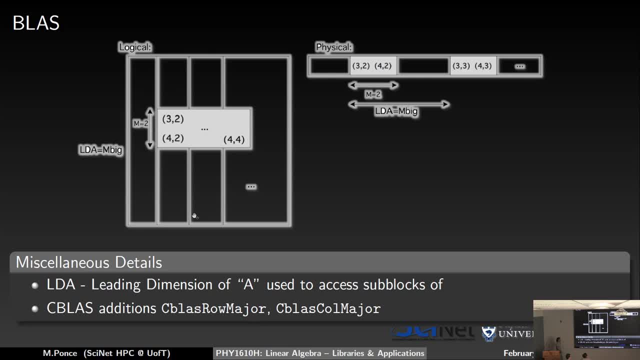 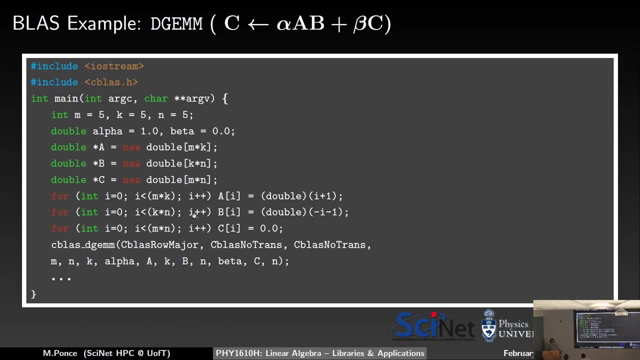 So picture is column major row, major plus. but if you really like both everything, It's a way just to fill some values in the matrix. You choose whatever, but you just choose something If you're working in Fortran. 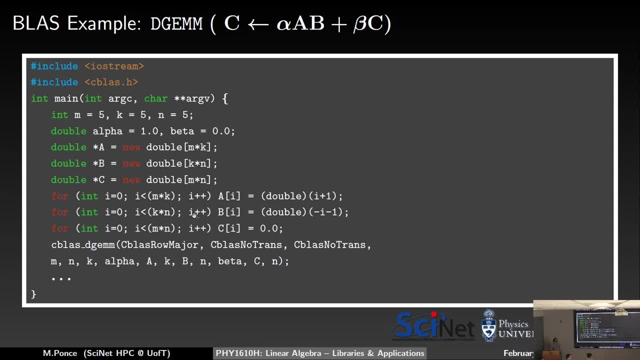 If I'm working in C, I'm calling Fortran function. Oh no, now you have to worry about all. So basically, everything that you think is one matrix is transposed. You have to well, or you have to transpose. 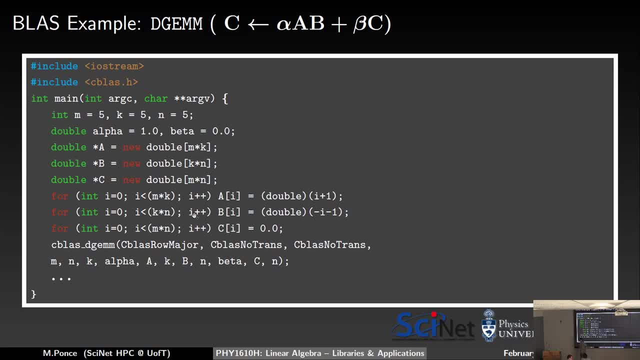 Yeah, But you have to think about all the time. Yeah, It gets tricky. We're using C function, Right So? So that's why these guys typically don't ask you for the major or for how it's stored. 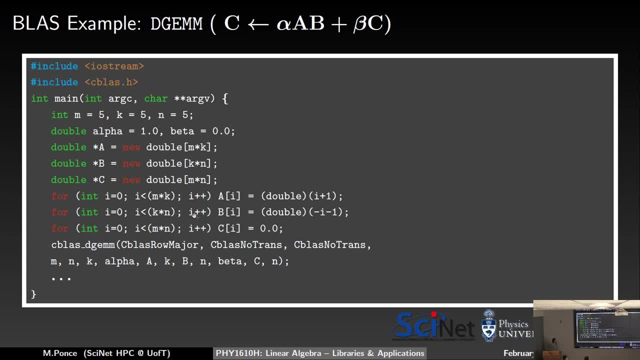 because they know that, at the end of the day, this C-blast on the 4D gem is calling the Fortran Like giving these flags. it'll just make sure that it'll So. this is how it looks, the output. 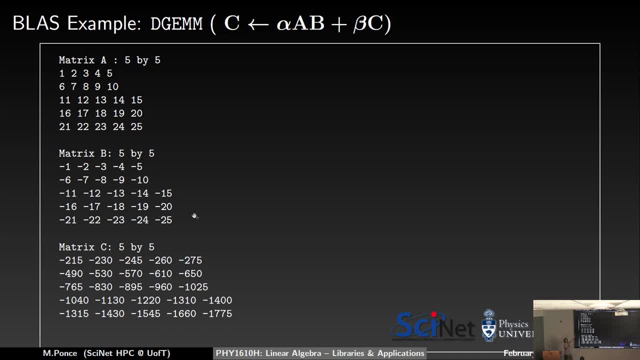 So that's the original matrix and these are the numbers that come from this: I plus 1, and minus, I minus 1.. And the matrix multiplication: Okay, So that's how you do matrix multiplication. So let's take a look at Lapec. 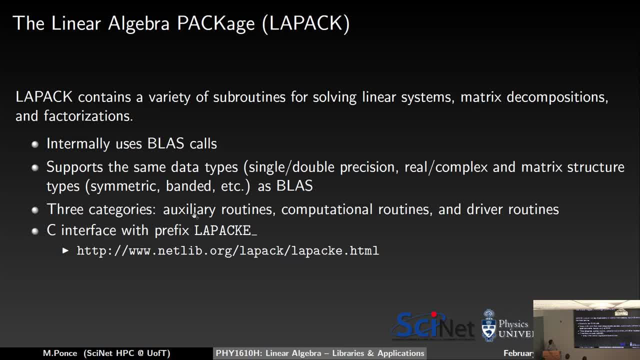 So let's see how to actually So. Lapec is the linear algebra package, So it contains this variety of solving, of solvers for linear systems, So let's take a look how to do that You can do also. it actually was something that is going to do while solving the linear system. 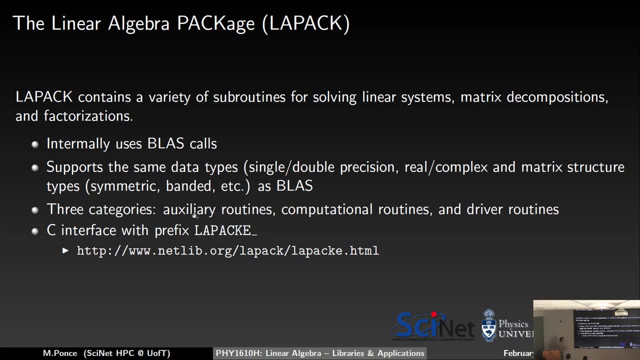 It's going to solve: doing this LU decompositing- So you can do the compositions that we discussed last class- and creating this pivoting matrix for reaching the lower-upper triangular matrix decomposition. Basically the nomenclature is the same as in BLAST. 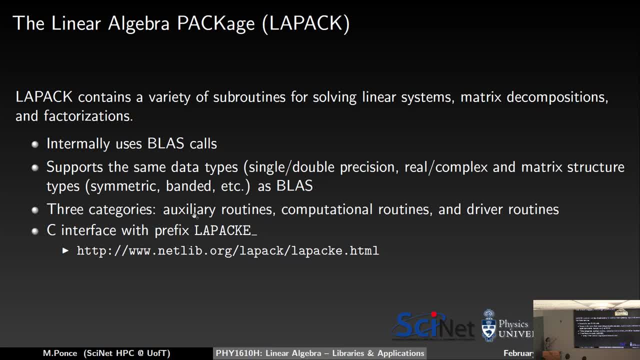 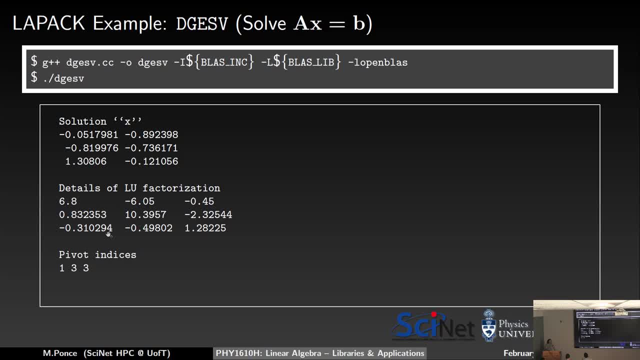 So there are actually three categories as well, like auxiliary, компьютasi, computational and red. So there are actually three categories as well, like auxiliary, computational and dry. So there are actually three categories as well, like auxiliary, computational and dry. 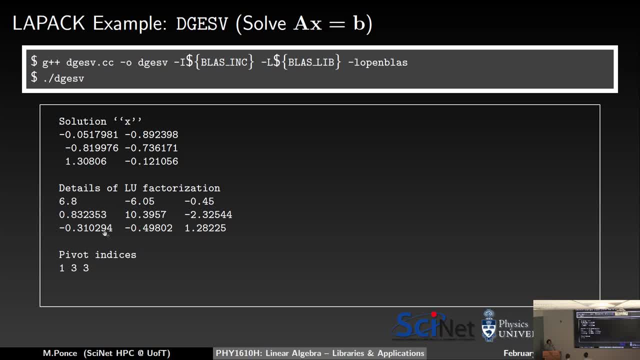 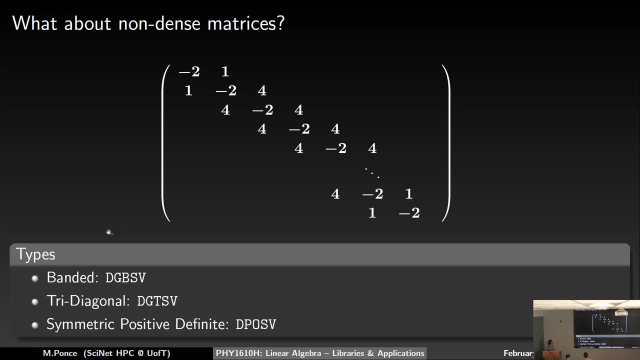 Okay, Do they all? Something has to do with 골�raf? No, this one is included right in the BLAST. I think: Okay, another class, okay. so what's about the this structure matrices like the banded matrices, or matrices that are non dense, so the ties that are associated with. 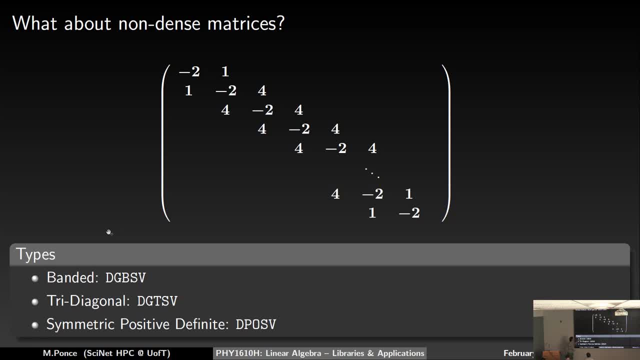 that other ties that we can use are banded matrices, like if you have like shots in the diagonals and soup sub diagonal. this one is very frequent and very useful because it's three diagonal, so that one already knows that you have the diagonal, upper and lower diagonal, and then we have- we may have- symmetric. 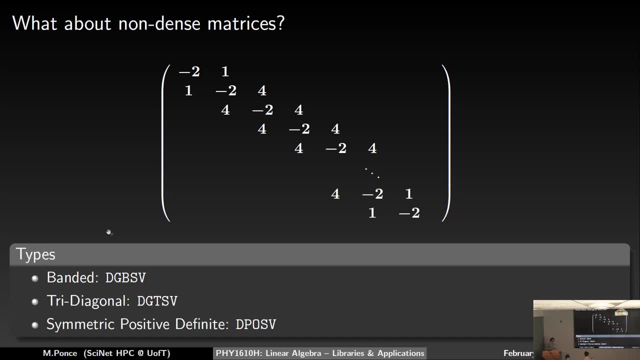 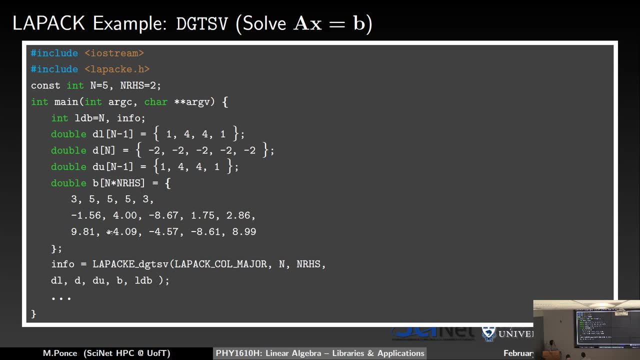 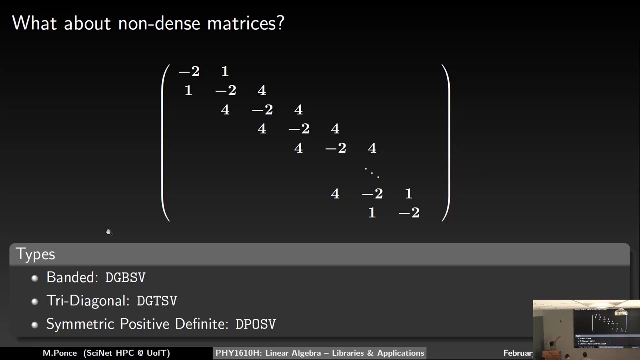 positive definite matrices, as we saw in last class. so how we deal with those? so let's take a sample again, solving a linear system, but in this case with the previous matrix, where it is is similar to the one that we saw for the PDS, but now this is has some force, probably higher order, the composition. so if 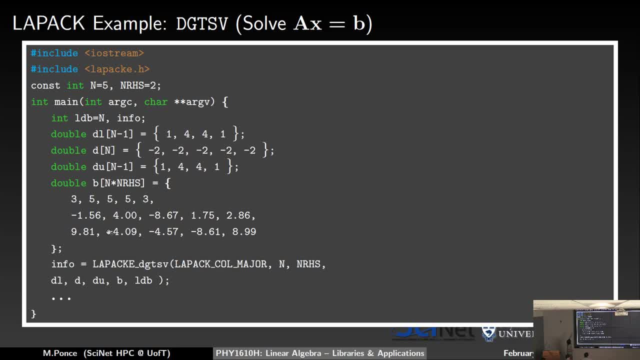 has one for four. so notice that. okay, we're going to use again Leipa key, we're going to use a five by five dimensions in this case and again, we're going to be solving for two vectors. so the number of Raja sizes two. this is a nice way of. 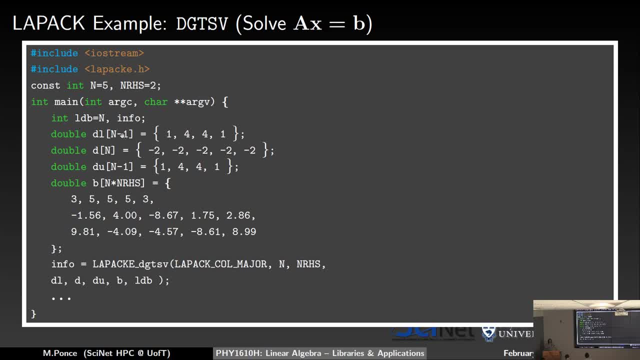 setting the leading dimension, so you don't need to worry too much. you always put equal to the dimension of the matrix. you are dealing with the whole matrix and that is it. so again we need the info flag for knowing the status of the of the solution. we define the lower diagonal with one less element. the diagonal has. 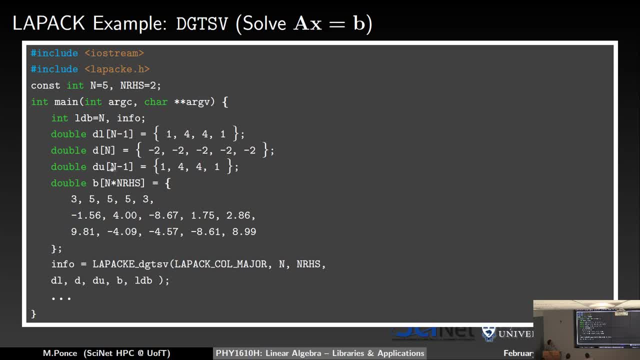 five elements, as the dimension of the matrix, and the upper diagonal as well, has one less element. okay, the vectors are actually three, not two, so this is a type of here. so we have three independent vectors, okay, so, whatever those are, and again, the only thing that we need to specify now instead of the DCE is this: is: 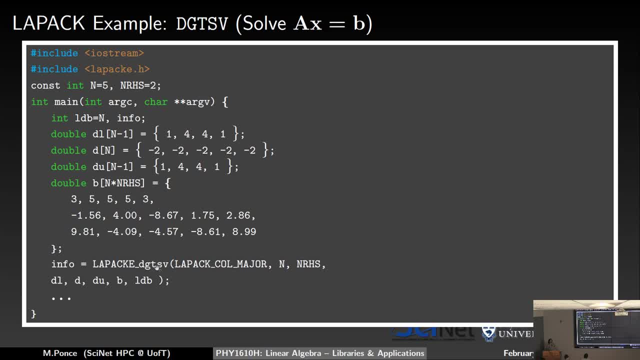 a triangular double share, a triangular symmetric matrix- sorry, banded matrix. so I can call the mayor number of dimensions run high side and now the, the difference that we specify, the three diagonals, lower diagonal, diagonal and upper diagonal, the vector of in the dependent terms and the leading dimension of the independent. 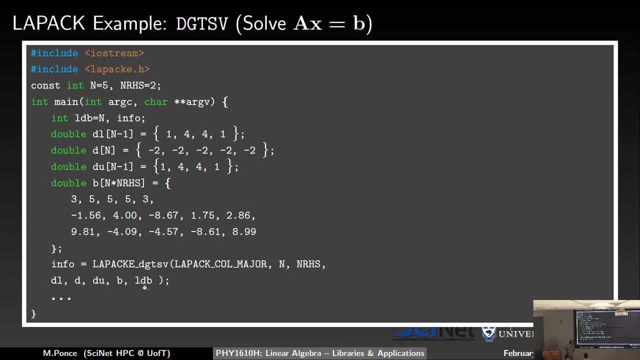 yep, so second, oh well, it will be nice to have it then- and dynamically located. it's just a matter of choice. he doesn't matter in the, in the, in the communication with the booster routine. yeah, initially I was lazy here, and so the compilation goes as before. 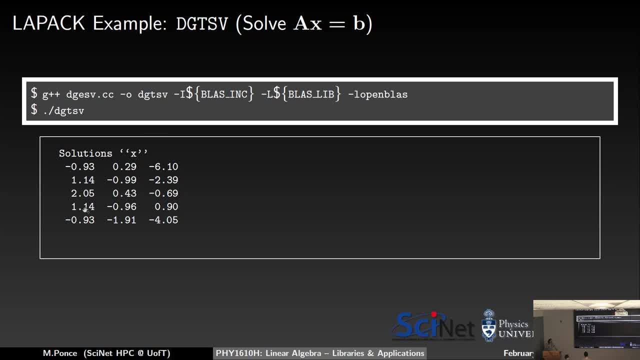 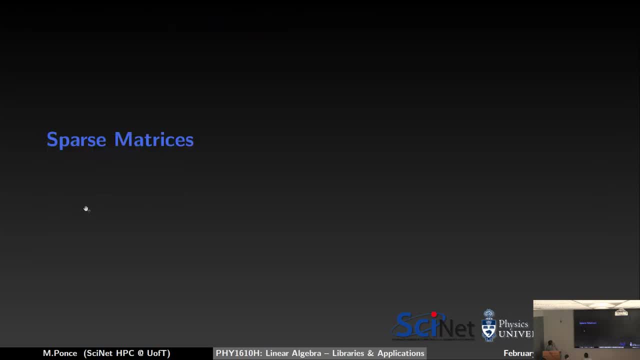 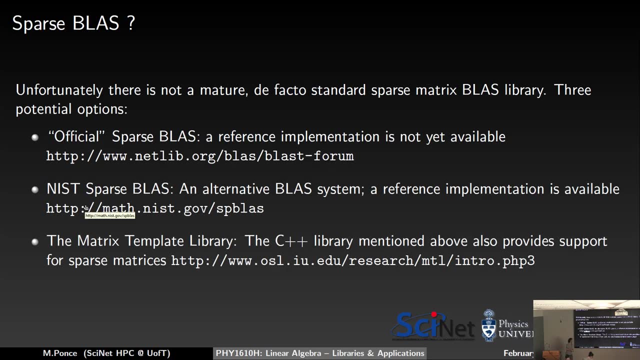 right? no, because every time that there is some more integrations, all changes happen. it has a new PAULMAT야 going to have three in the pendant vertus. what about ania, sparse matrices we talk a bit about, then. the truth is that there is no official implementation of sparse matrices. there is a sparse blast or a nice sparse blast. 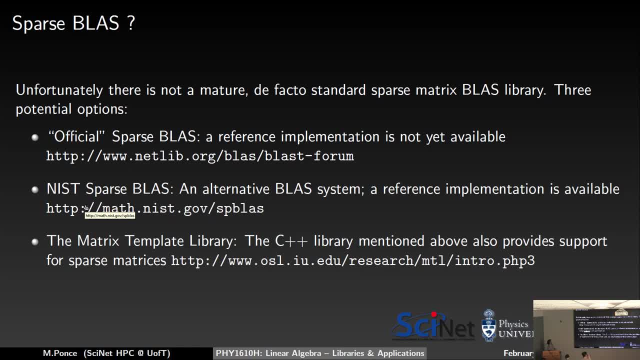 I think the matrix template library may have something, but ok, maybe instrument is not even balls very well and I cannot give the Matteo. my question is: is this a these fall ekam words where Mitt listen to data you because you write a little moment about this not gonna work, but what you're learning is you look at this. 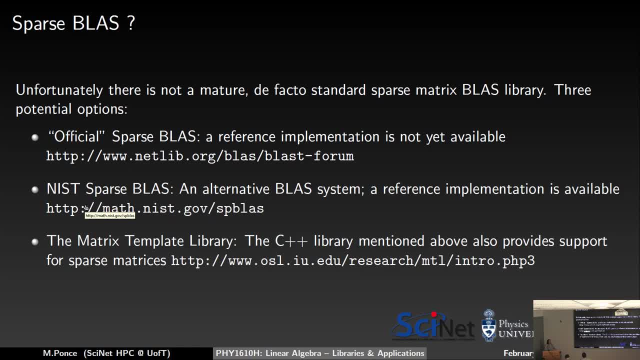 there need to learn what I mean with each other before you know this. dollars for the, But there are no standards, as there are for the other, for more general matrices. But there are some reference there if you want to take a look. What else? 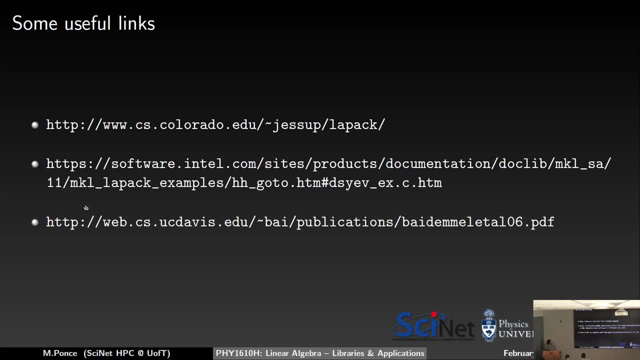 So these are some useful references again if you want to deal in particular well, if you're using something from MKL, this is a very interesting link for taking a look. But then these other ones are just for the standard implementations of layback. 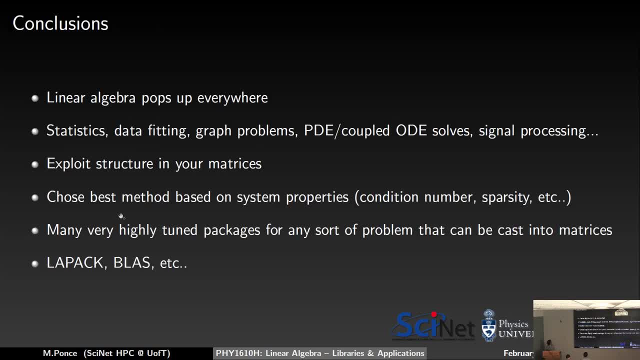 and blast. And well, I think the conclusions is like the same: as we have been mentioning and hammering: you guys Try to use these libraries, try to get familiar to them, with them, Try to exploit the structure of your matrices. In the problem, I think we have a 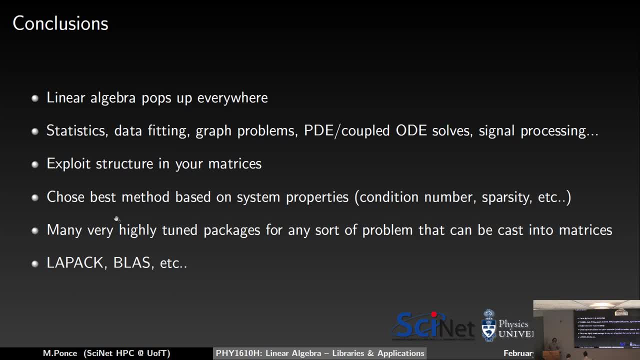 thing is positive symmetric matrix. so whatever implementation you just try to use, that's underlying the routines that you are going to use. Yeah, Choose your functions accordingly to the structure of the matrix that you have. Okay, I think this is it for today. 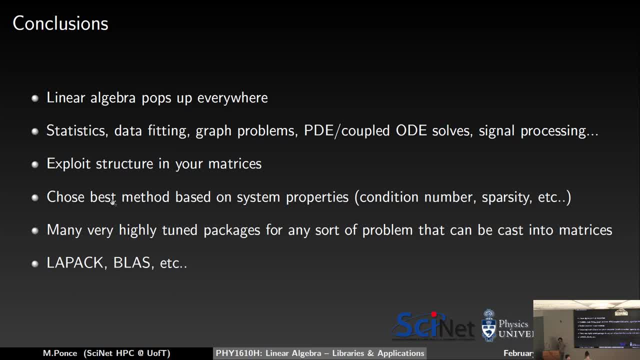 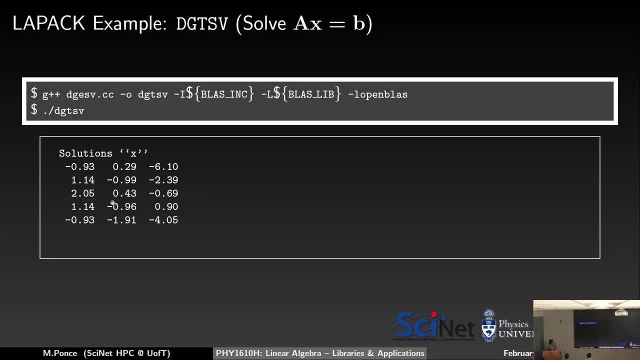 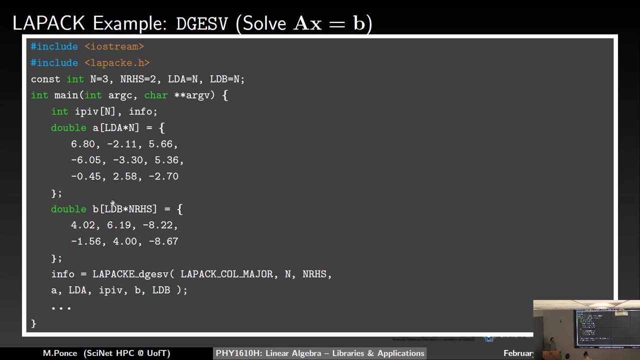 Any questions? Maybe with the dimensions and all these examples, all the matrices, for some reason we're all one, Yep, Yeah, Yeah. So that is odd, right, And it's very on C, or even on C plus plus C. 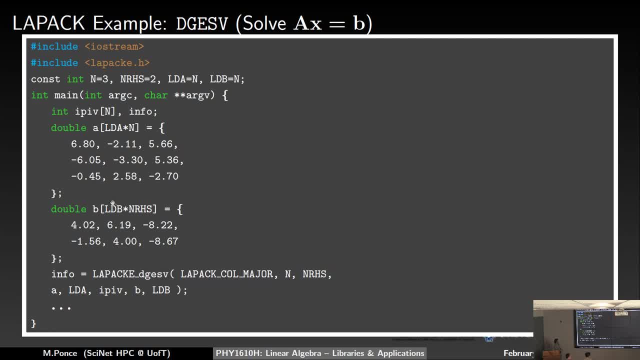 How are these made? They're just vectors. So, because you specify what leading otherwise, in other words, where the next row starts, these routines know that this is a matrix. every time you pass an element, The routines layback and blast. 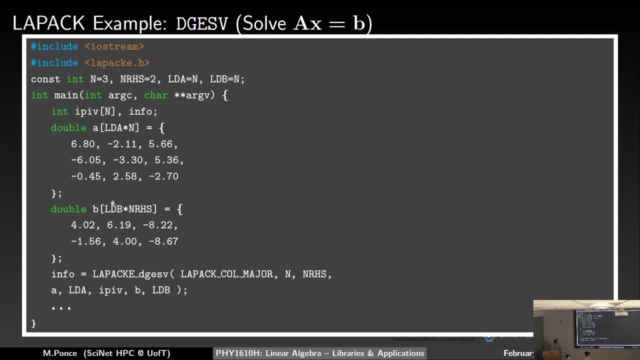 only care about the fact that these are now contiguous in memory or skipped by a lead, So they can anticipate, then you're when you're using any other package than in your arrays, So for instance, dimensional arrays in C or C plus. 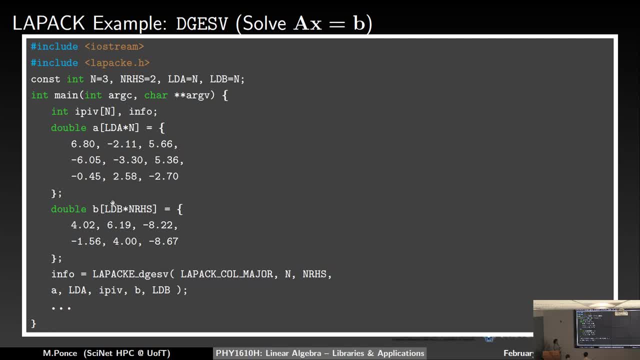 again are arrayed, Just to make sure that those matrices are have continuous elements, that if row one is in here, row two is in somewhere that it is So we've seen in the array even just using C plus. 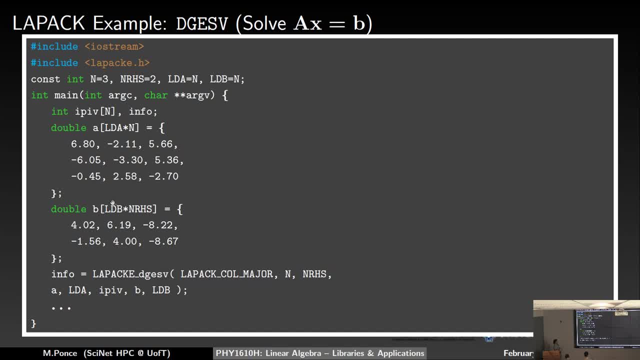 there's two ways: one where you allocate rows and one where you allocate rows one at a time, and one where you block the latter one. every layout. First one, you'll find text laid back. This is how you create a dimensional array. 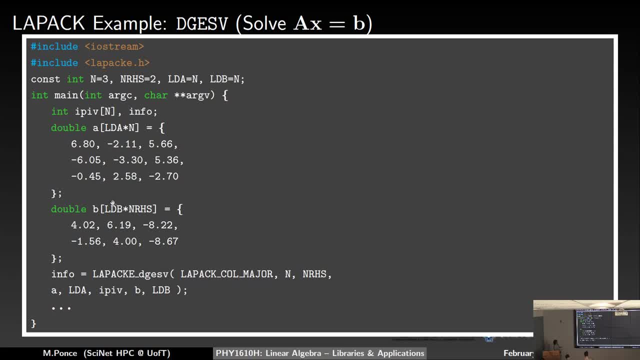 that dimensional array will come. So it has a warning And that's why all these, all these samples just using a flat layout of the of the array, And how bizarre They array by time and everything Is this dimensional. 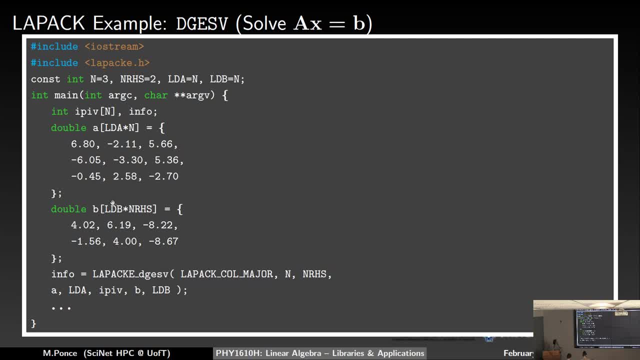 Well, it depends how it's laid out. You know, in Fortran it's columns and so Oh yeah, yeah, So yeah, it's a. it's an off concept, but it makes it. I mean. 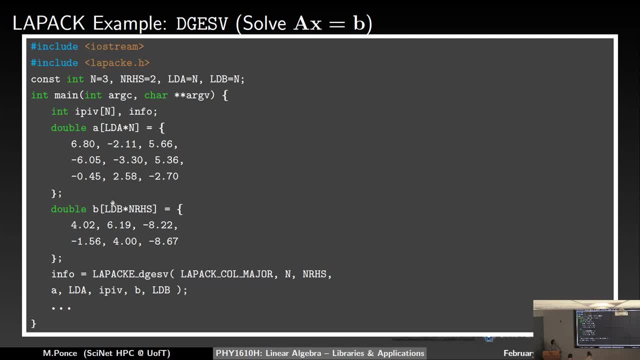 it makes sub matrices possible. Don't have sub matrices. LDA is going to be your, your own column. Okay, This is a bit of like a general question, because I've done a bit of that stuff in Python and I know that Python, at the end of the day, 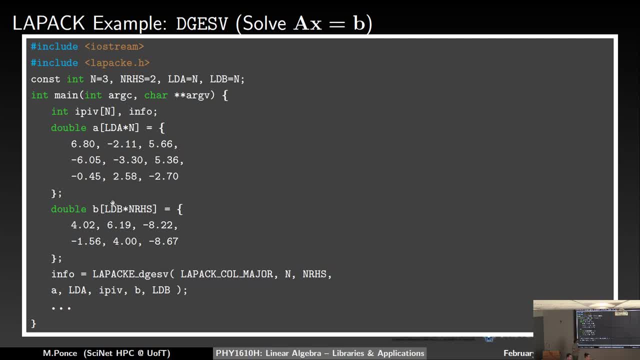 is also used in, But it's much simpler, however, to code it right. So I was just going to ask, like: is there an actual advantage like doing things in C plus? I don't know, maybe I'm. 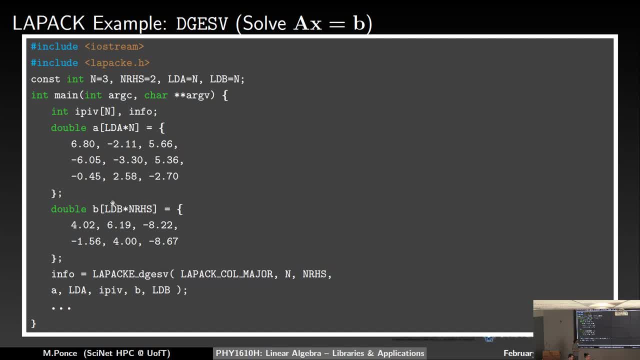 maybe I'm missing the point in some specific aspect, just because everything is using a lot of So, But in in terms of Python you mean Compare C plus plus with Python You can use CYCLE. That's the last one. 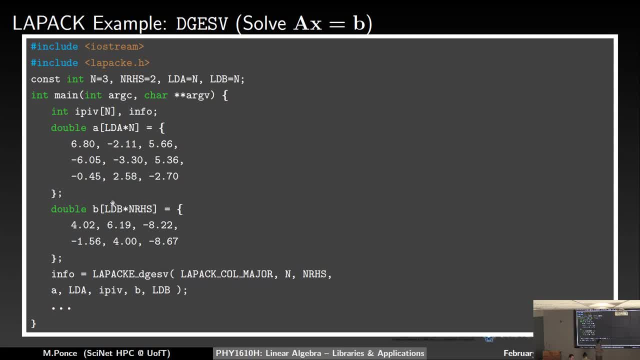 Well, I mean something like when you're using, let's say, noun y. as far as I know, it's really doing everything here like C or right, But there's still. Yes, that's true once you're at the laid back level. 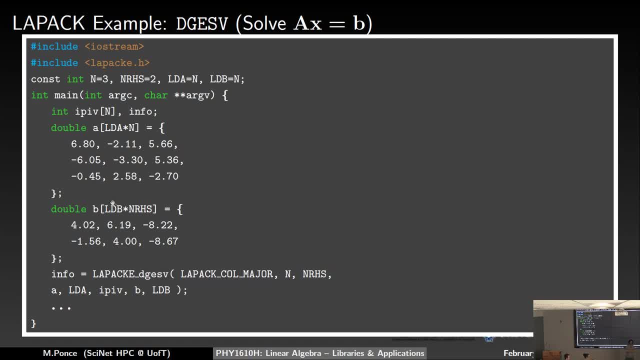 but everything else you do right. So you're still in the laid back in your data reading, the file still on that side. I would still have to look at your script line by line. has to figure out for every variable. 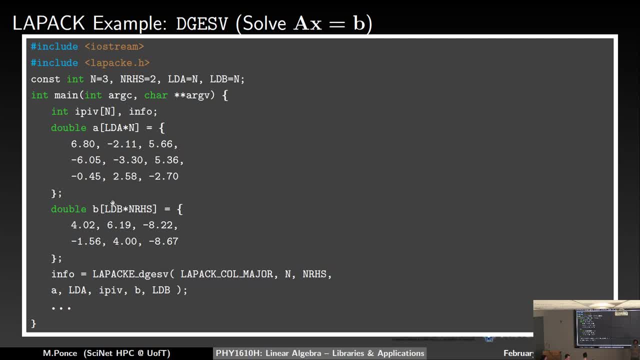 what its type is, has to basically distinguish which type it is, which laid back, routine call, And so there's overhead. There's still a little overhead, so it So if the majority of your stuff is spent in a laid back or blast call. 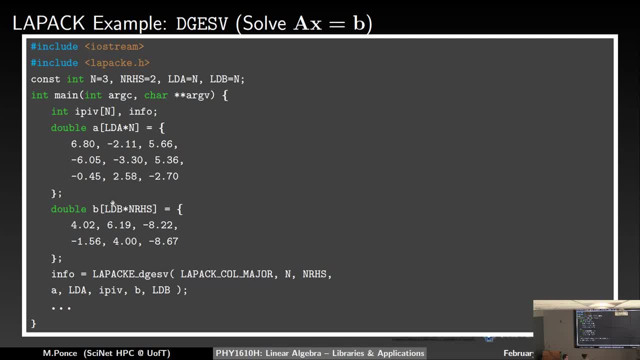 you're right, Then it doesn't matter, Right, And? But if there's a good bit of other stuff going on is then we'll see. The other thing that's harder to do, I guess, is There are also things that the compiler can do for you. 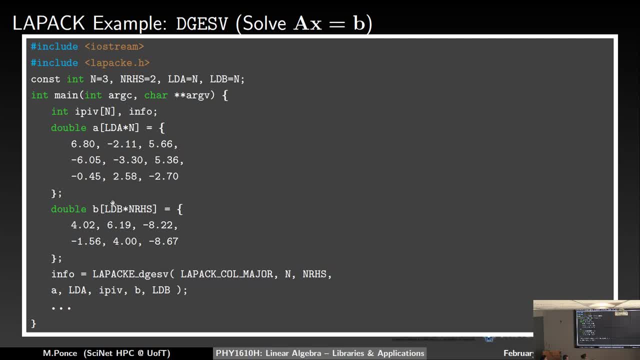 right. This thing of having defined the variables and the and specifying the types not only makes the compilation faster, but also allows the compiler to reshuffle and reorder things, especially if you are using a level of optimization three, which is quite aggressive. 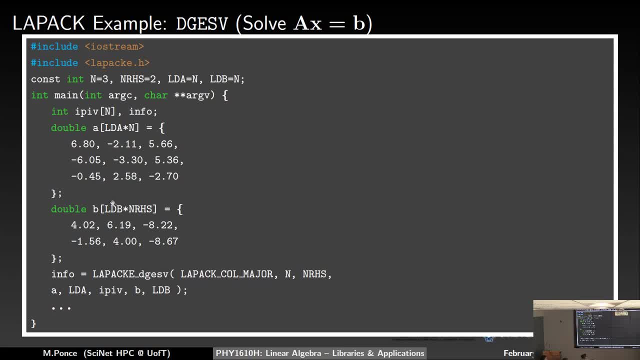 So it can reorder instructions, just to make it run faster. So back to the Cython suggestion. If you just take your Python code as is and you run it through Cython, it's not going to be any faster than Cython. 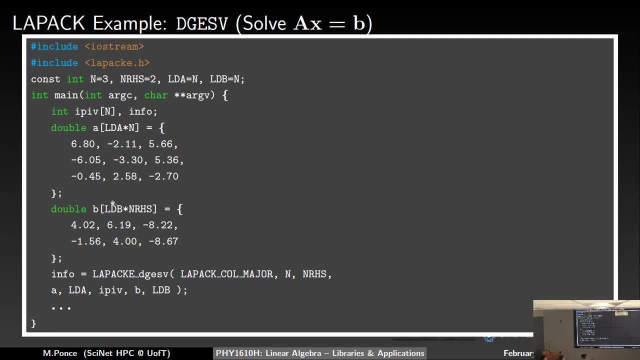 But, as you mentioned, for Python or Cython, so what it should be doing in C, then yes, you could. So you're still going halfway. Sometimes it's a good way, but if you know you're going to be performing sensitive